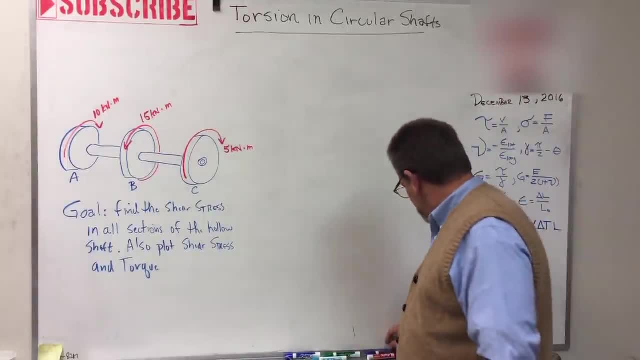 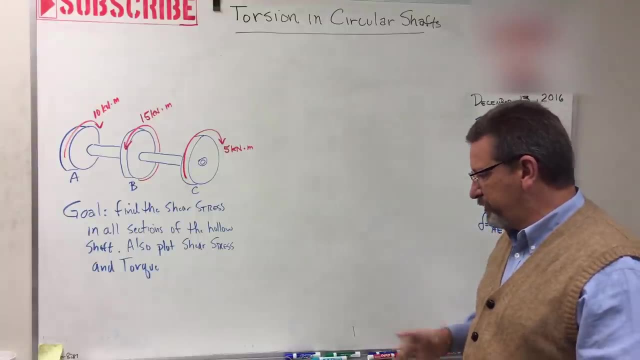 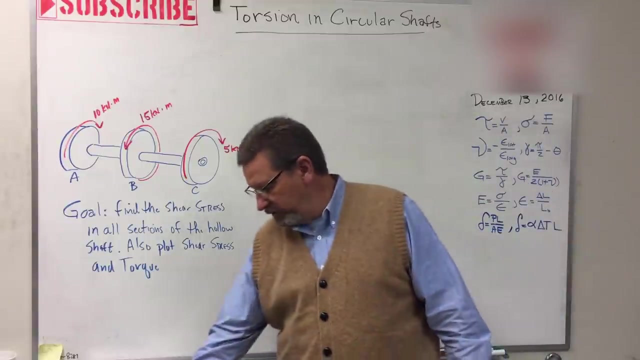 Hello friends, It's time today to talk about torque. We're going to talk about torsion and circular shafts. It's kind of the next section in the book. One of the things we're going to talk about is, if you have a circular shaft, look a pool noodle. 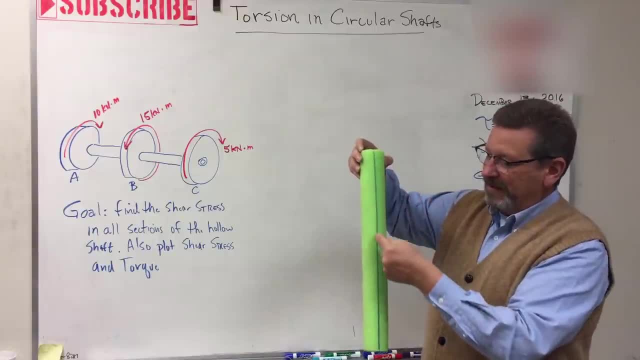 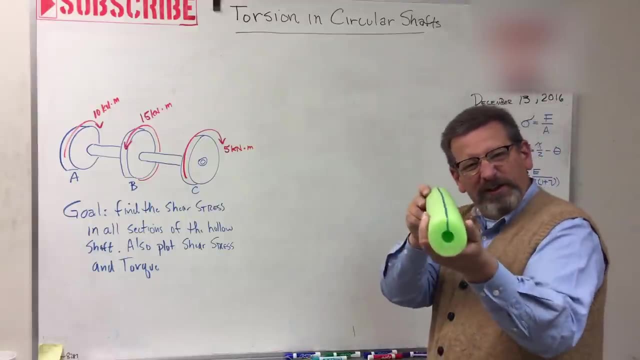 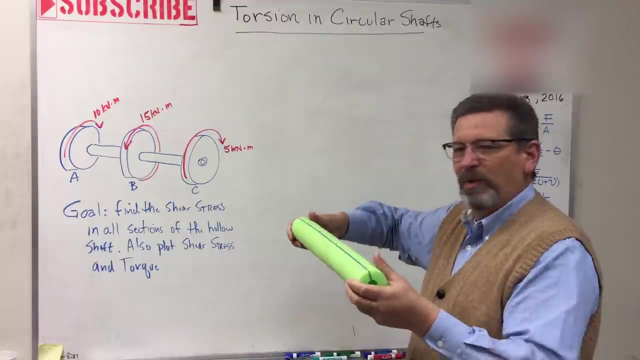 It's a good example of a shaft. I have drawn a line down the middle of my shaft, here this beam, And I've also put a line here on the end. So let's call that 12 o'clock, right? So what happens when you start twisting on beams? right, If I twist one end one way and the other end the other way, I apply a torque, right. 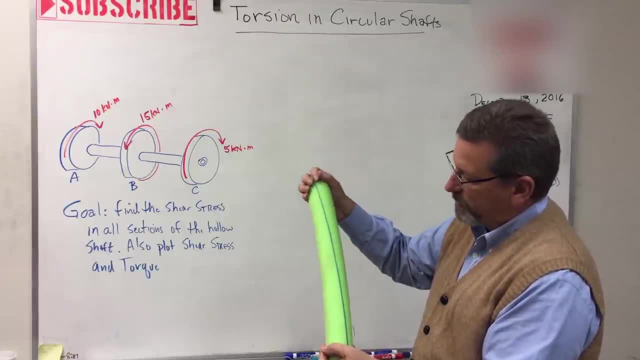 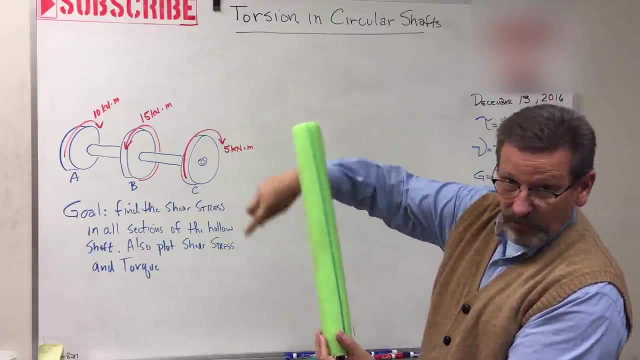 What's going to happen to that straight line? So, as I apply opposite torques, look what happens to that straight line. Is it straight anymore? It's kind of helical right. It kind of wraps around the beam. And also, if I hold this end still and twist just one, 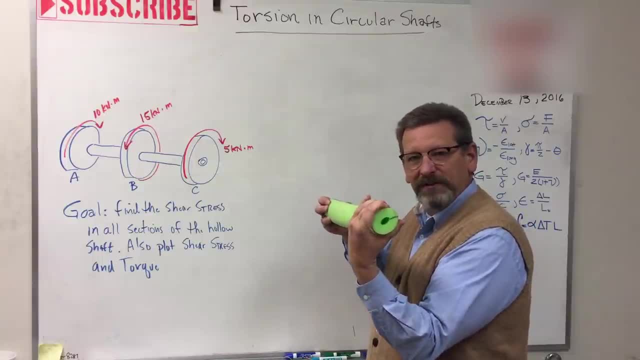 If I hold this end still and twist just one end that 12 o'clock mark, what's going to happen when I twist it? Is it at 12 o'clock anymore? No, And that's called the angle of twist. okay. 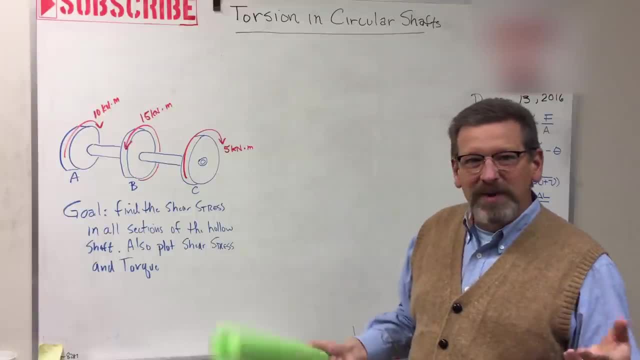 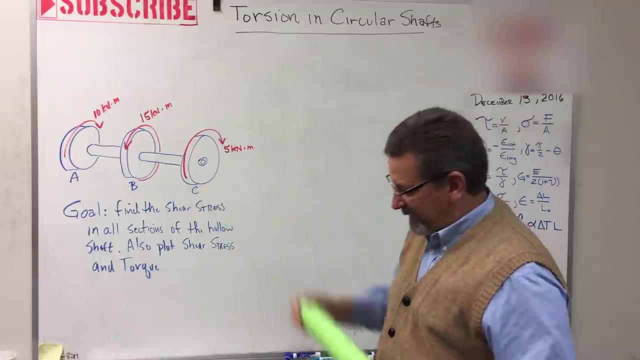 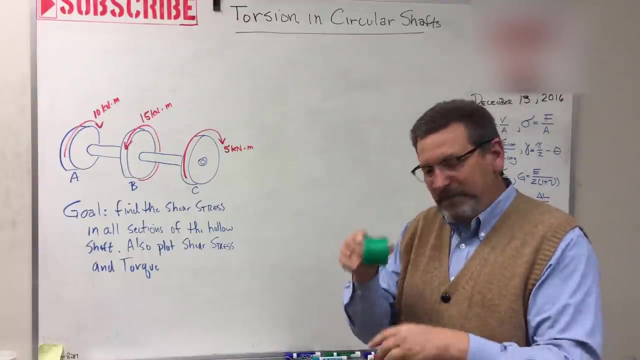 And there'll be a video coming here right down the road that'll tell you how to calculate that angle of twist. But what's going on as I twist on a beam and I start torquing it like that? What's going on? Let's go back to our slinky here. Let's think about a beam. Here's the same beam, a little section of my noodle beam. 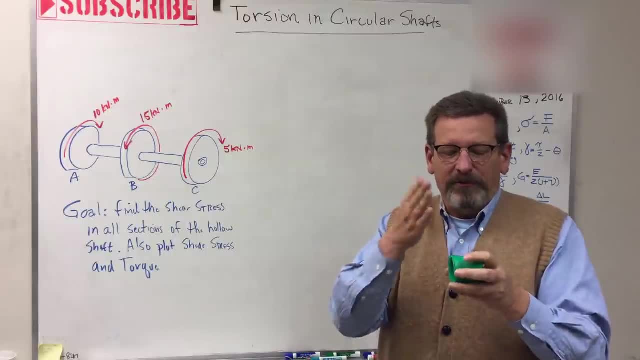 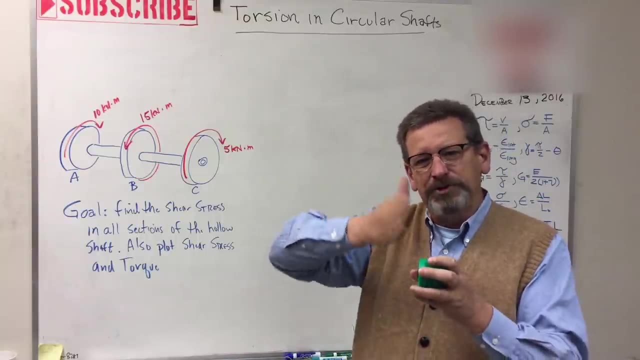 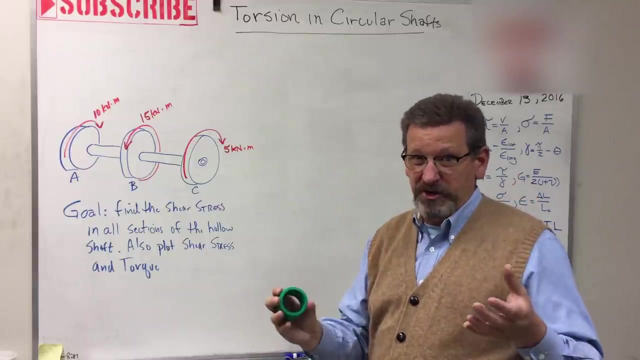 But as I twist that, what's happening? Well, think about that beam having little planes in there, little shear planes. right, As I twist that beam, those little shear planes are sliding one relative to the next one, okay, And so we get torsional shear, okay. And what is shear stress? Do you remember? 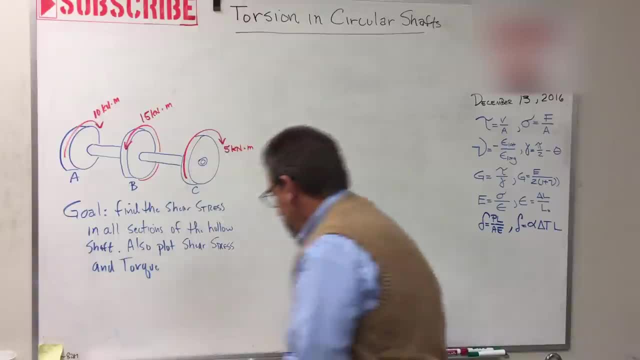 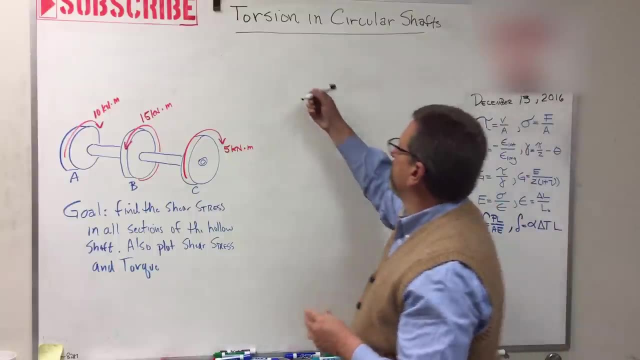 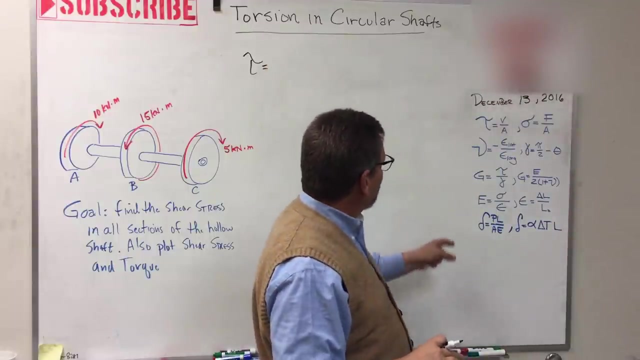 Yes, we remember, because you told us that already. Remember shear stress is. I have a lot of markers, So I'm going to show you what shear stress is. Shear stress is given by tau. okay, Now remember we talked about tau before. let's look on our little list over here. Do you see a tau? There's a tau. 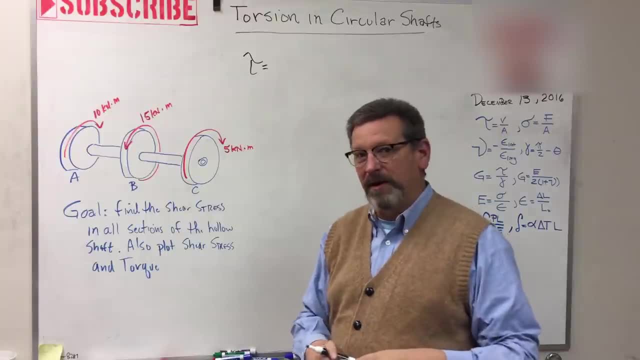 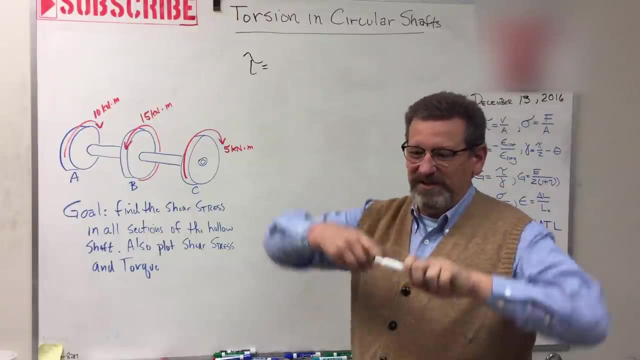 Right, it was V over A, and that's when I had a beam and I was trying to tear it apart that way. right, It was the force, the shear force, divided by the cross-sectional area. Well, this is a different deal, right, Because this is shear due to torsion. okay, So a totally different kind of shear. 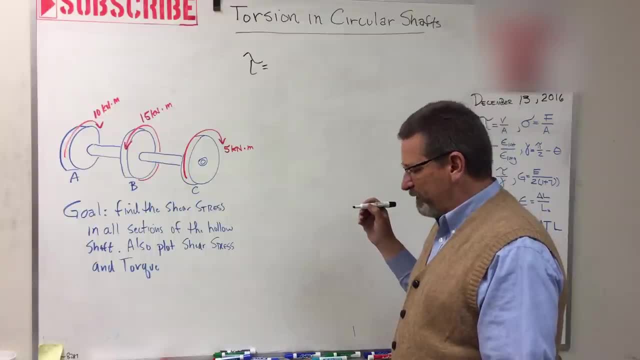 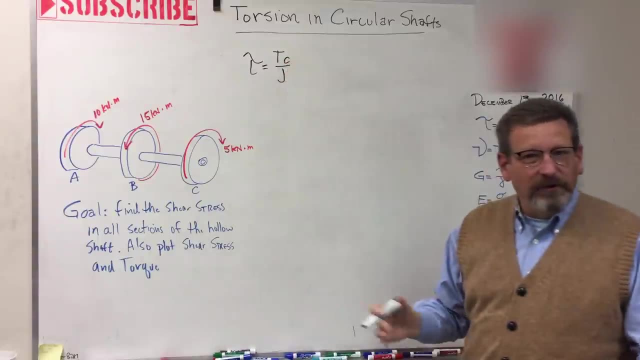 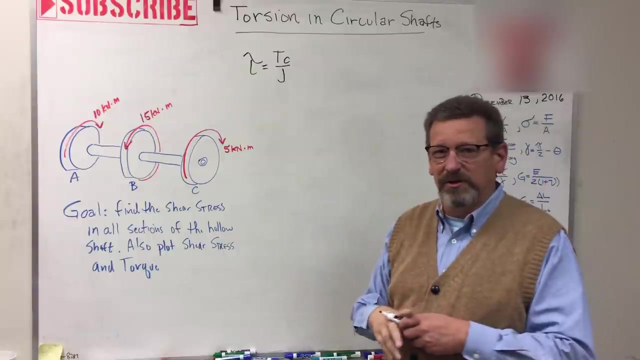 Okay, is going to be a little bit different. We have a different equation and that equation is this: Tc over J. So that will tell us how to calculate the shear stress in a circular shaft when it has a torsional load applied to it. Now, on a torsional load like that, if I twist that like this, 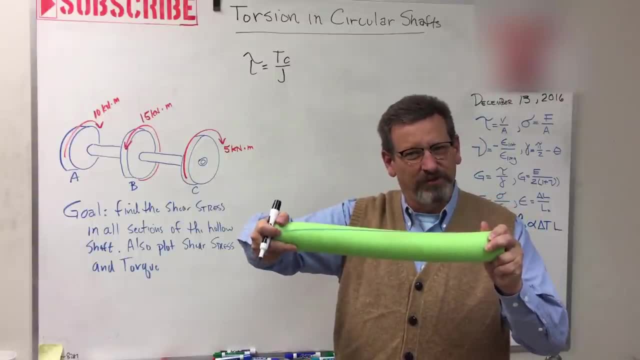 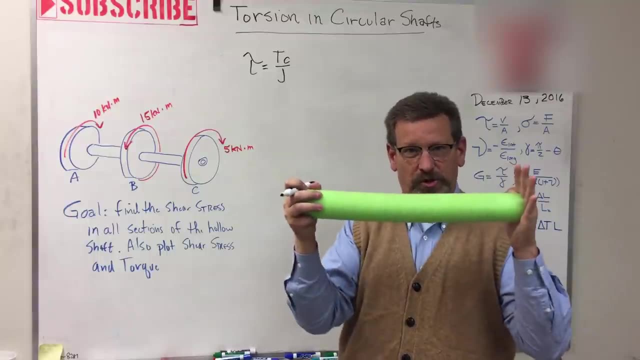 do I ever have sigma stress? Am I going to have normal stress? Let's see what was normal stress? That was, the stress by it was either trying to make it longer or shorter, right, but just twisting it doesn't cause sigma stress, does it? So I'm not going to have sigma stress here, or? 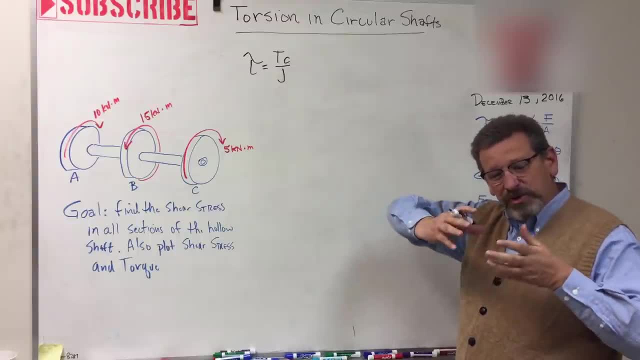 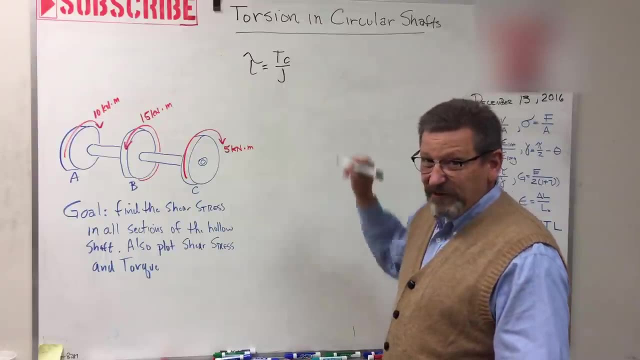 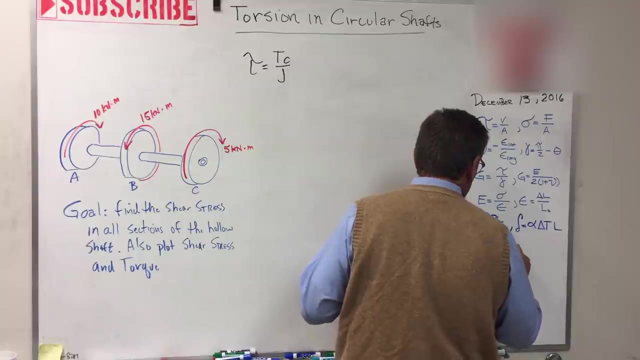 normal stress. I'm only going to have that shear stress where it's trying to shear along that beam. one plane to the next. okay, those imaginary planes. So that is a new equation for our list over here. We'll have to put them on here. Let's put him on here. Tau equals Tc over J. 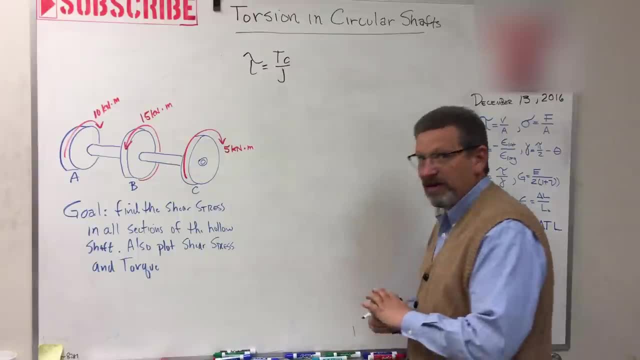 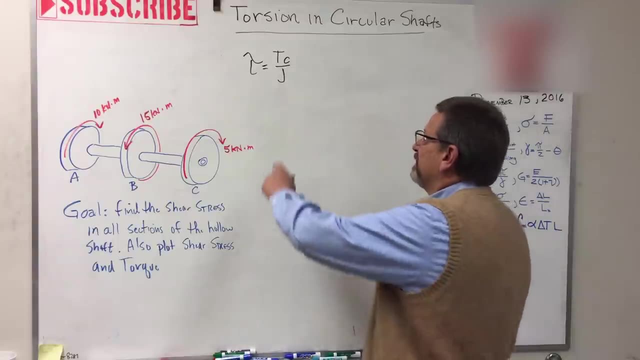 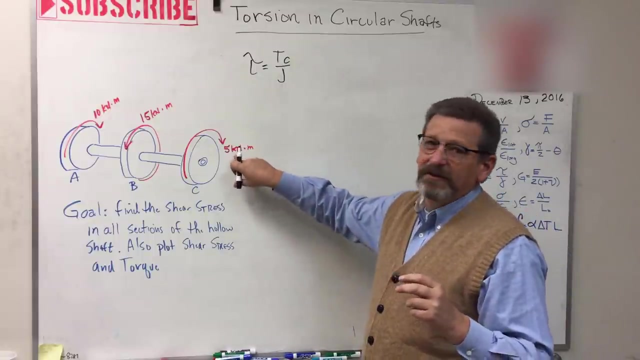 over j? All right, new equation. I told you we're going to have a bunch, So what does this mean? Okay, so tau is shear stress. We know what shear stress is. What is T? Capital T? It's not time, It's not temperature, It must be. what is that? Torque, right, Torque? 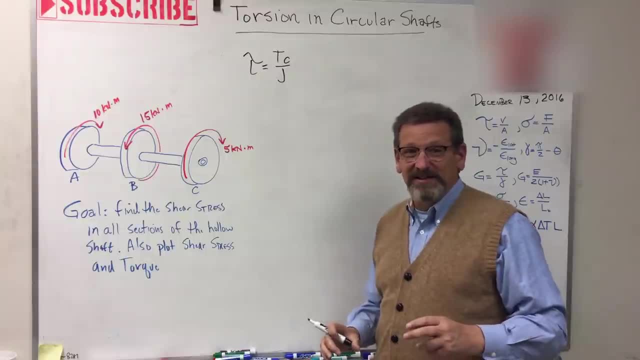 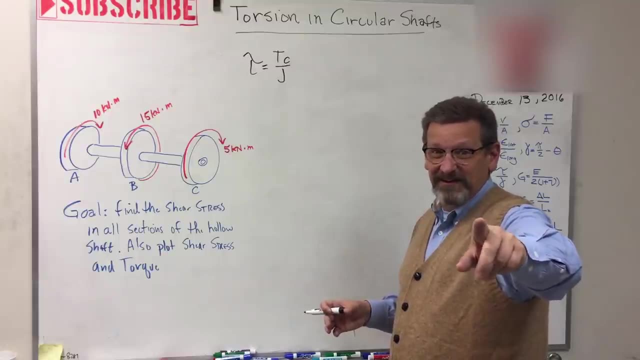 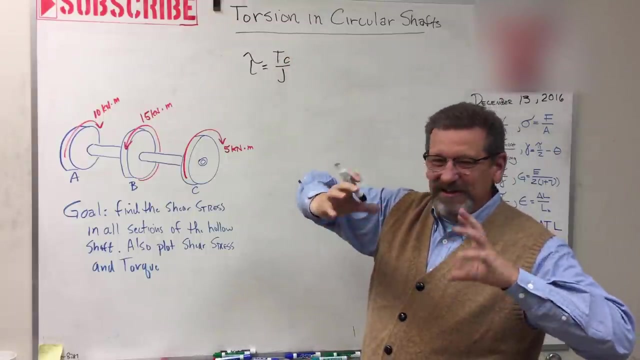 is nothing more than a moment. You want to trick your little buddies there when they say, hey, what's torque? You say just a moment And leave them hanging. Get it. Okay, it's a bad joke, All right. so torque is a force times a distance, right, It's a tendency to. 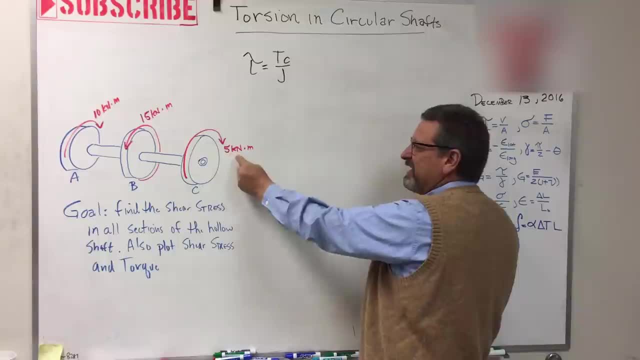 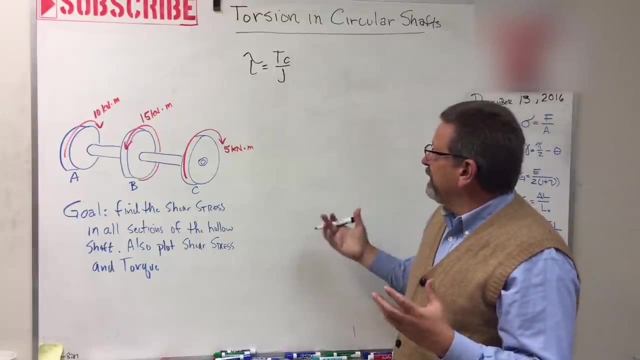 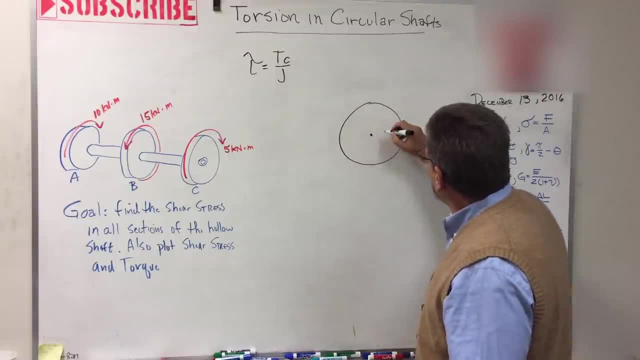 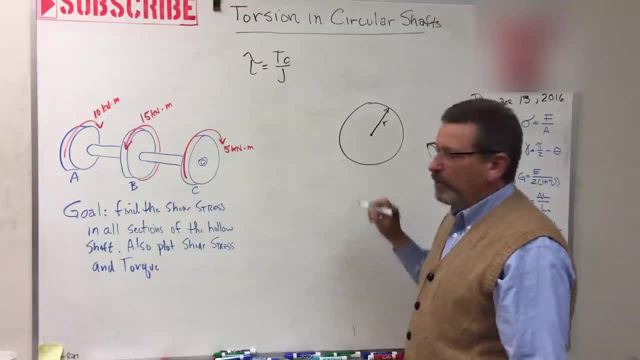 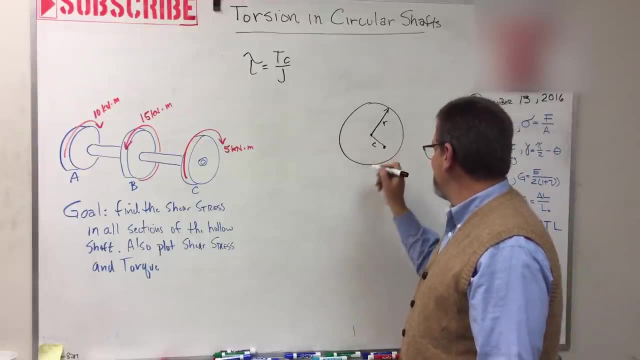 on at the outside, Because that would be R, right? What if I wanted to know what the shear stress was at that point? Well then, it's not R there, It's just C. It's some distance from the middle to the point of interest, right? And why would I want that? Well, for. 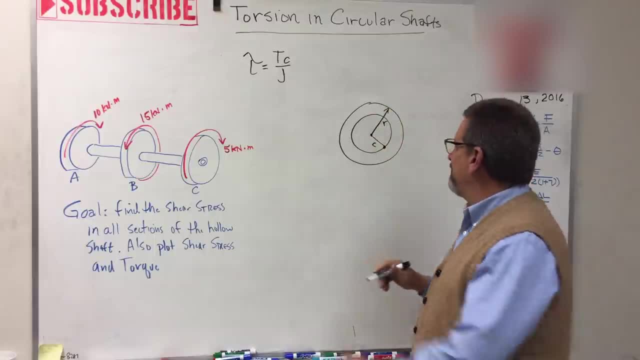 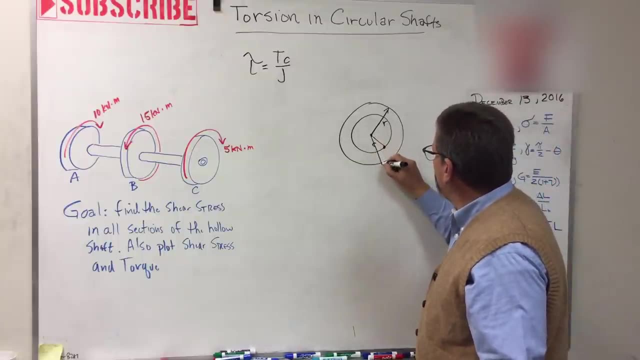 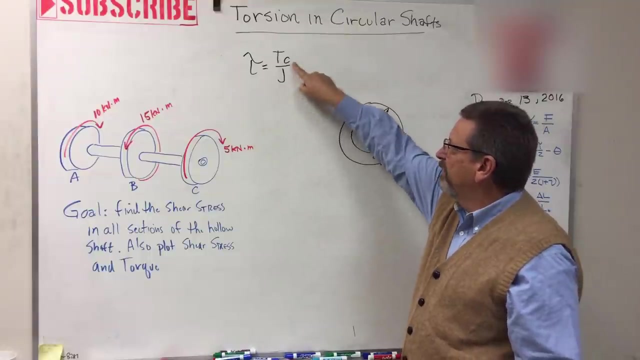 instance, if I had a hollow shaft, maybe I'm interested in the shear stress on the inside of the shaft. Now, looking at this equation though, if that's C or that's C right, either one of those is C. which one is going to give the biggest tau? Well, if that's on the top, 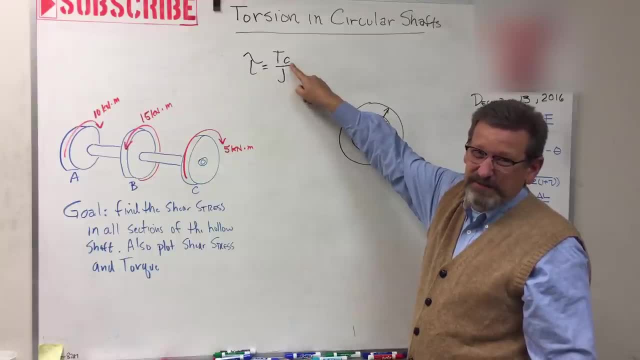 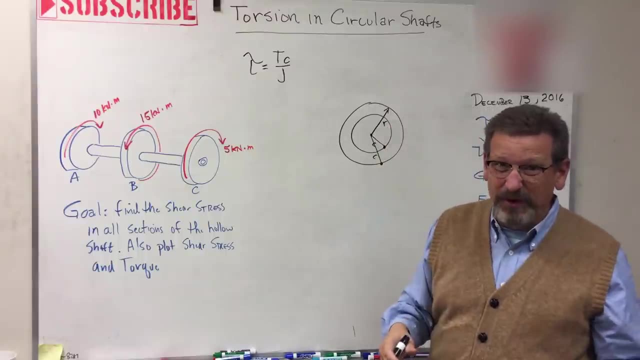 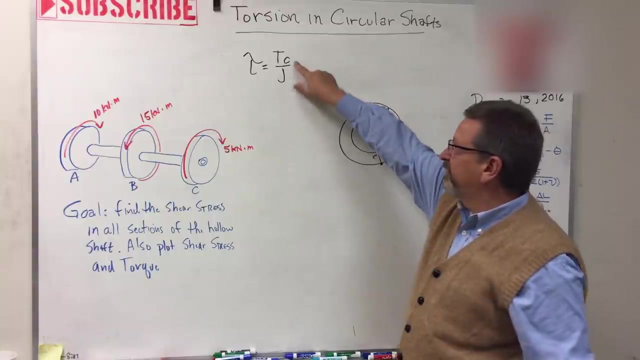 if I want tau to be as big as it can be, I need C to be as big as it can be. So what does that tell me? That the shear stress in the very middle, where C is zero, is equal to what Zero right? And the shear stress at the outside of the part? that's as far. 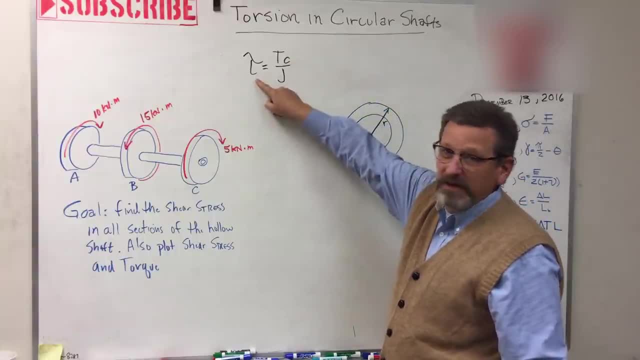 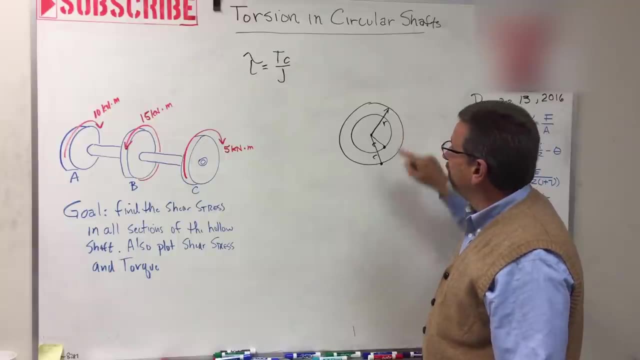 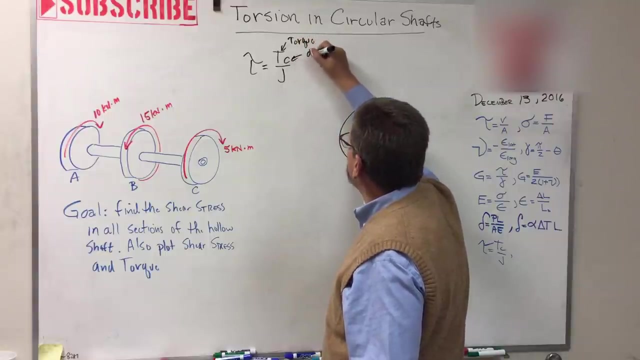 away as I can get. that's where the shear stress is going to be maxed. So shear stress goes from zero to max on the outside of the part, okay, So T is torque, torque, Q, C is just distance. okay, from the middle of the part to the point of interest, whether that's. 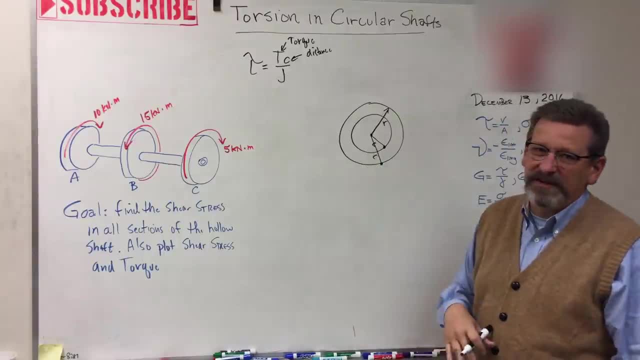 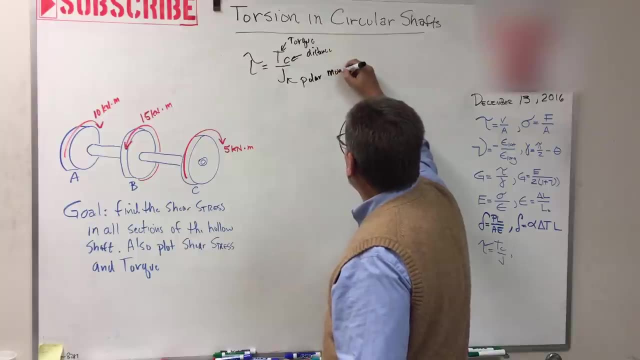 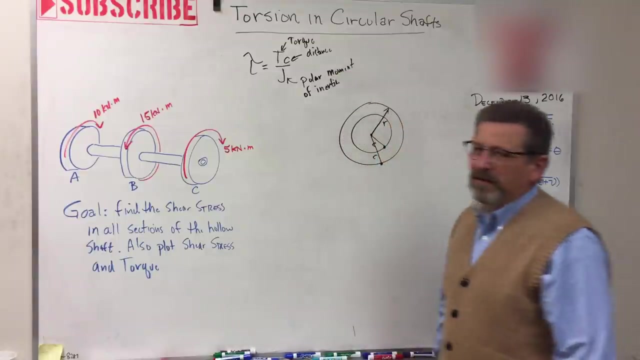 on the inside of the circle or the outside. Again, max is always going to be on the outside. And then J. What is J? That's called the polar moment of inertia, Inertia, okay. So what is the polar moment of inertia? What's the difference between that and capital I, which was the 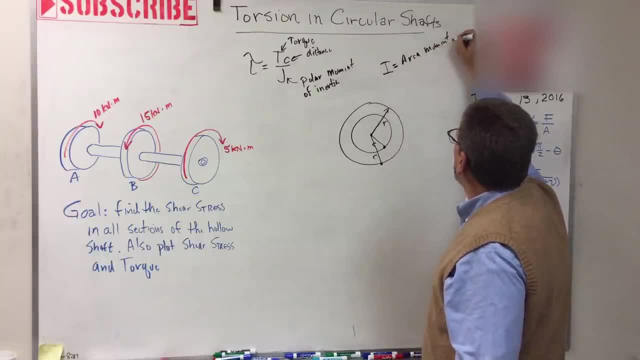 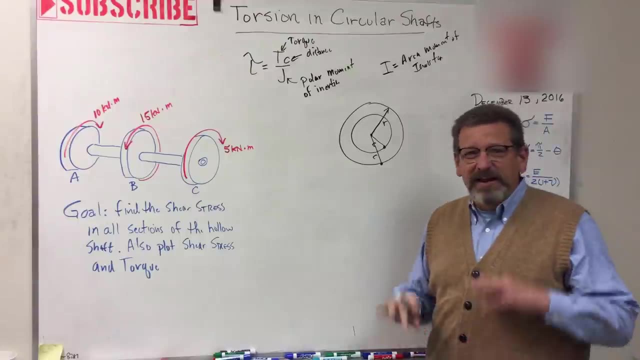 area moment of inertia. okay, Well, the area moment of inertia told us that the polar moment of inertia is no longer paper, It's the surrounding area And in particular, we see in general here there are four of our gains here, But we know what is the polar moment of inertia. 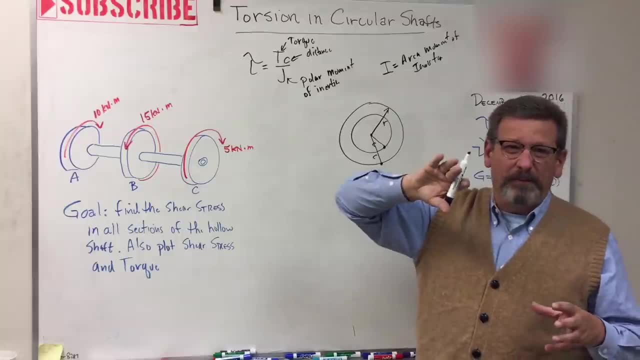 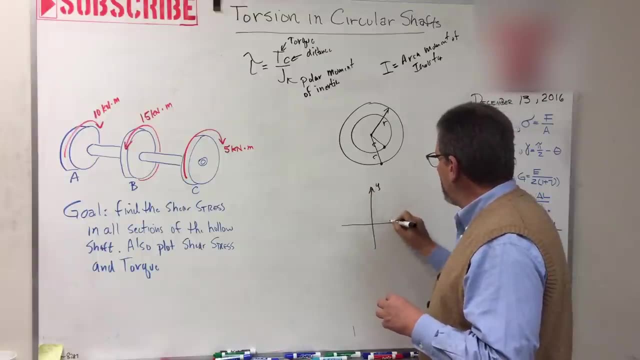 Like there is a polar moment of inertia, that this result was a resolution, So that's all this eats up. But then we go ontolly here and the this excess of inertia, the polar moment of inertia. you know the polar moment of inertia in Win küre case. let's say we're. 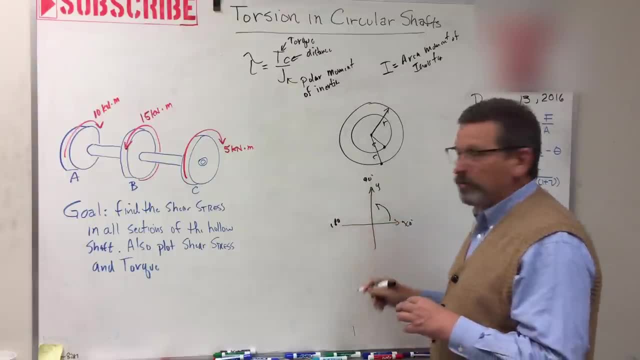 talking about half on the one side and these aren't to the right, etc. but this is a polar moment of inertia. How resistant a beam is to bending. And actually that's Chapter 6.. In the next chapter we're going to talk about that some more. So J The polar moment of inertia. 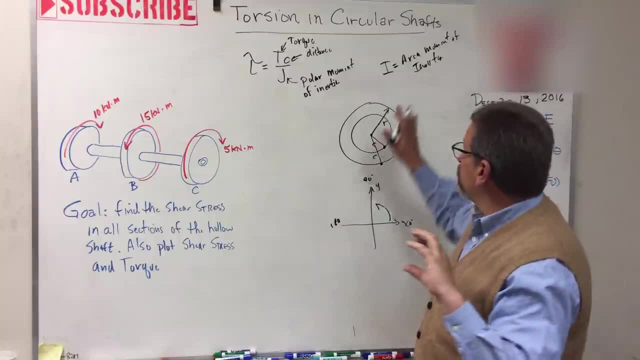 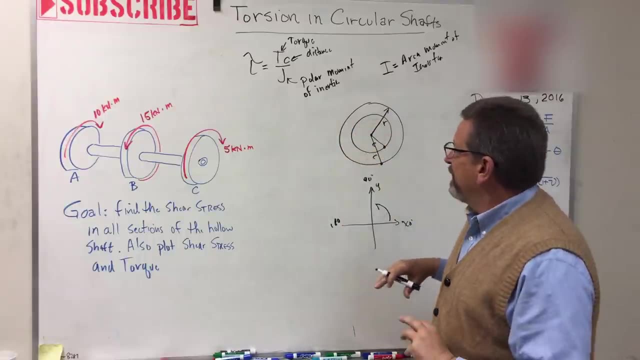 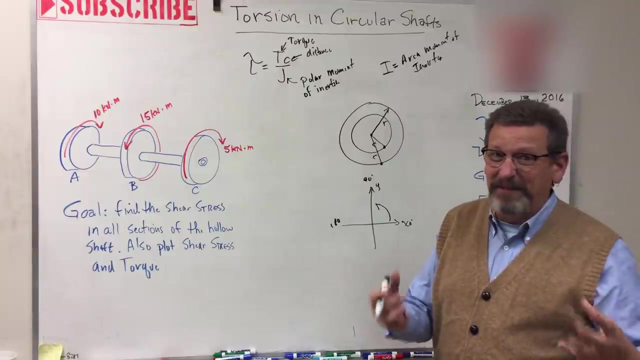 And remember, polar is a, remember, this was a polar coordinate system. right, This is X. and the resistance, where this was the resistance to bending, this is the resistance to torsion or twisting. okay, and the bigger J is, the more resistant that beam is going to be to want. 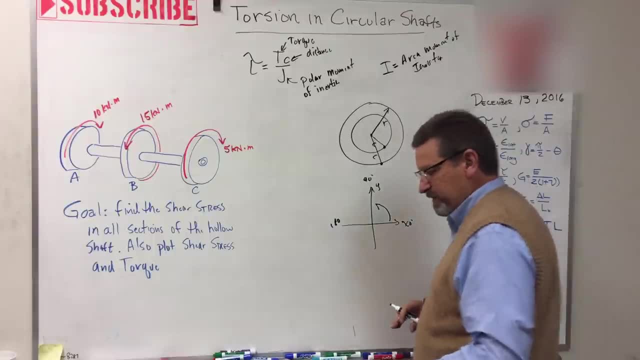 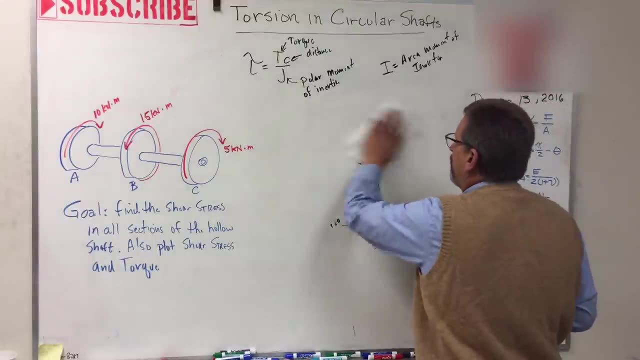 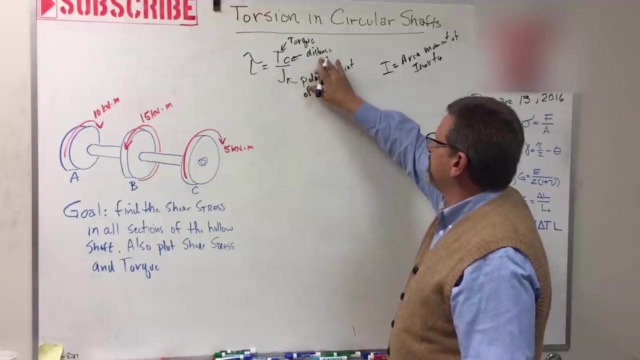 to twist right. that angle of twist is going to be smaller, the shear stress is going to be smaller. okay, I can't keep up with my eraser. okay, so we know this equation. this is a new equation force. we know how to find torque. it's just given, distance is easy, but what is polar moment of? 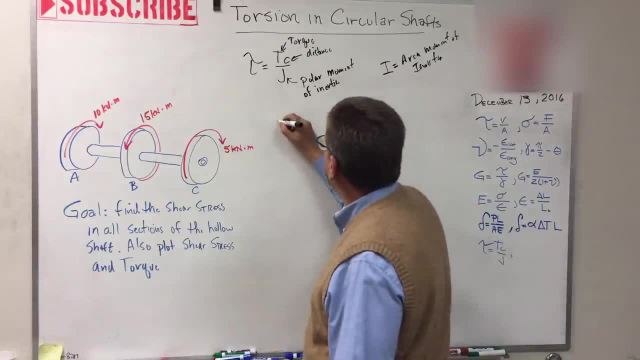 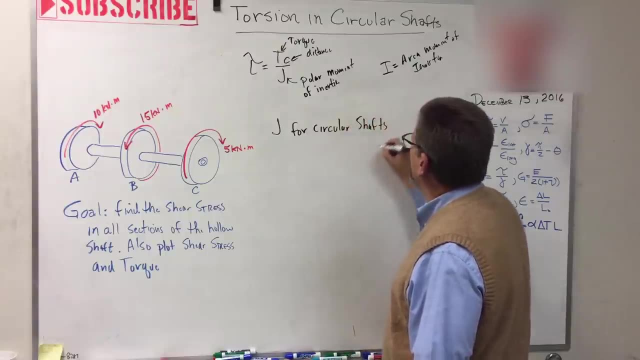 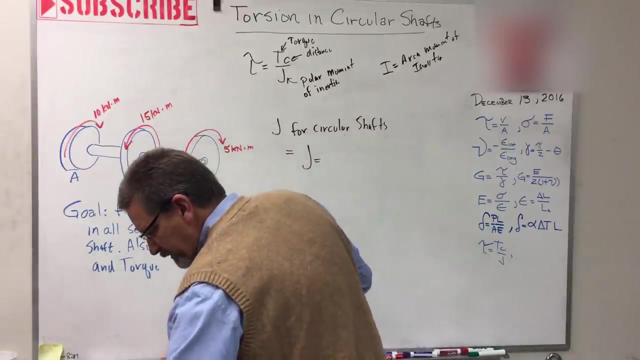 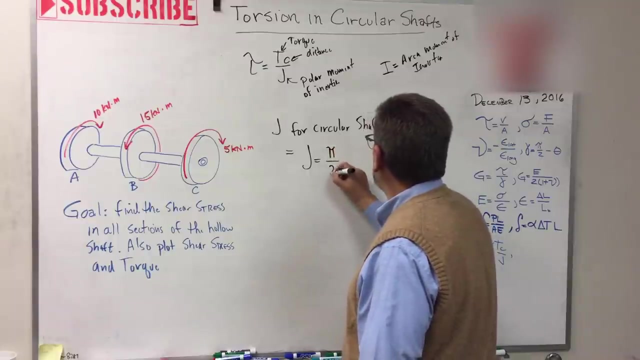 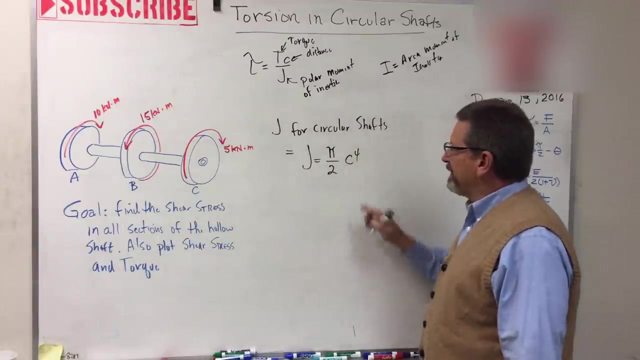 inertia. okay. so for circular shafts: okay, so J for circular shafts is equal to. okay, here we go. J is equal to. I have to look it up because I can't remember. okay, I know what kind of what it is. it's hard to remember. okay, it is pi over two times C to the fourth. okay, and that's going to be the outside. 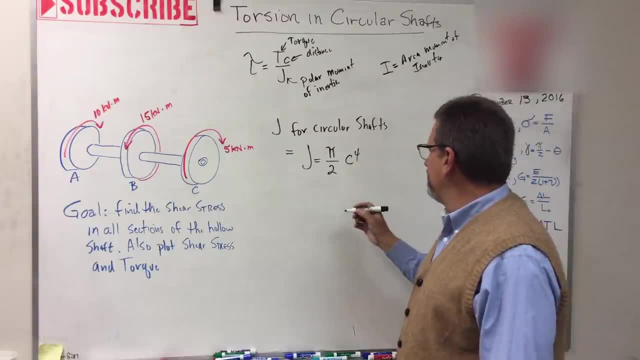 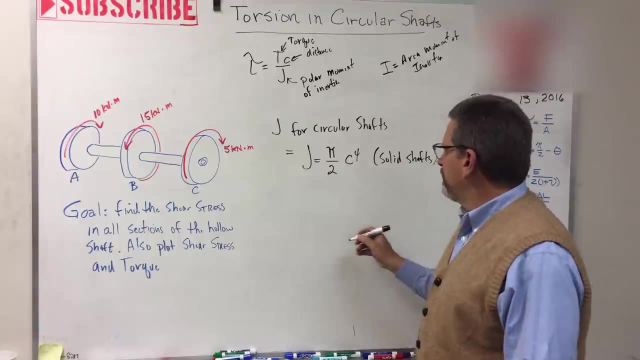 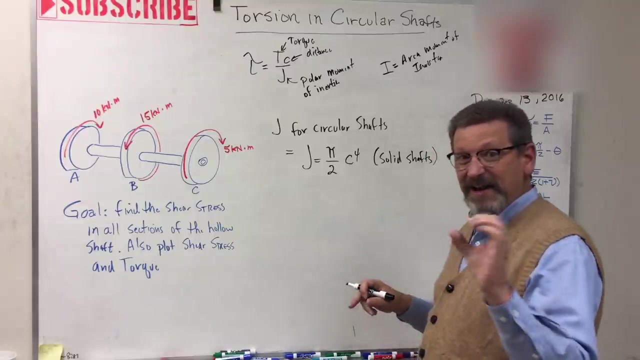 radius. right, that's the outside radius, and then. so this is for solid shafts. okay, for hollow shafts. Now, this one we're going to work here in a minute has a hollow shaft, It has an OD and it has an ID: an outside diameter and an inside diameter. 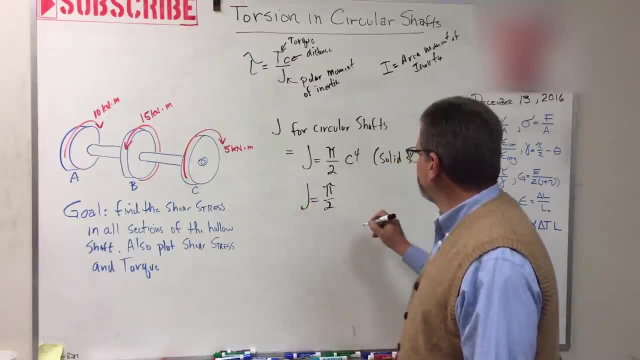 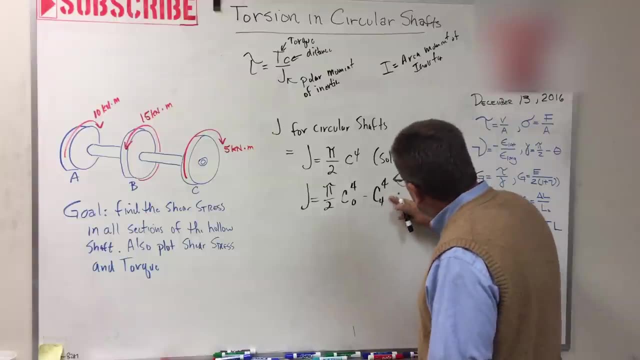 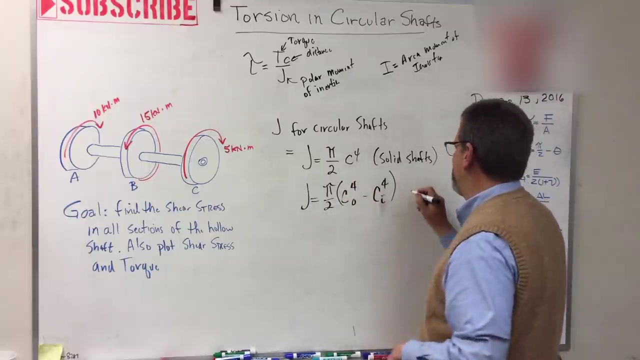 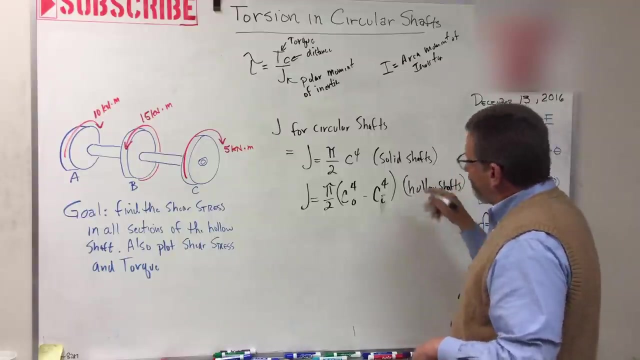 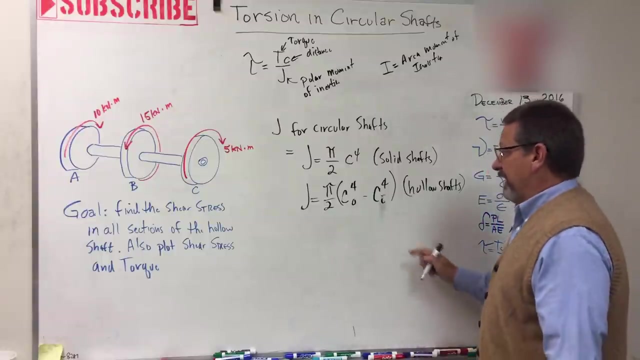 That is J equals pi over 2 times C to the fourth outside, minus C to the fourth to the fourth yikes inside. So this is the outside diameter, this is the inside diameter, And that's for hollow shafts. Again, these two equations are in your equation sheet that you hopefully will get on the test. 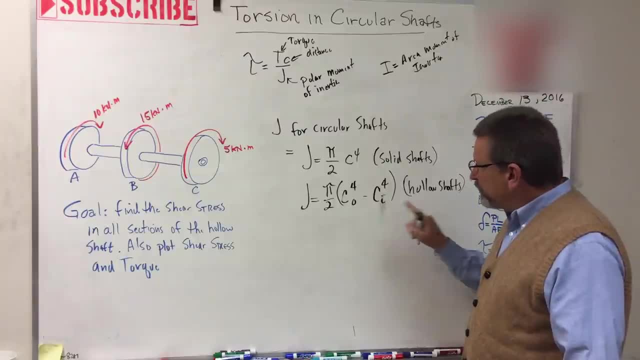 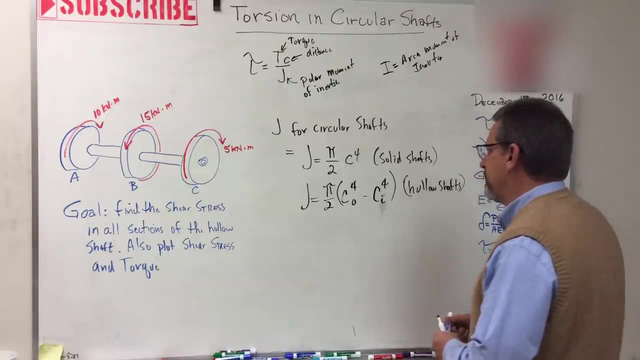 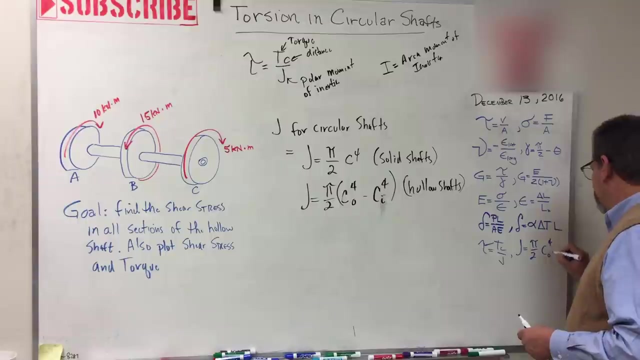 I hope you do. I would give my students these problems on the test. So that's two more things that we need to remember. So let's see, let's put those over here. So J is equal to pi over 2. C to the fourth for solid, and J equals pi over 2, C to the fourth outside, minus C to 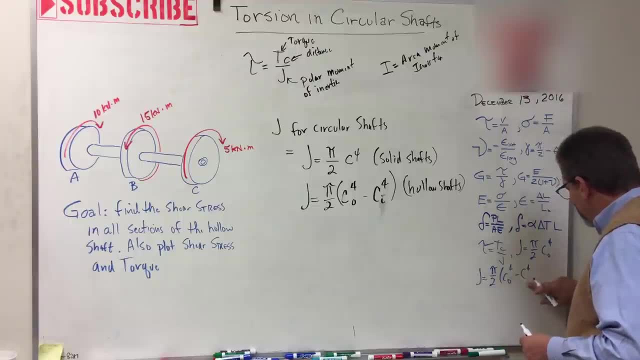 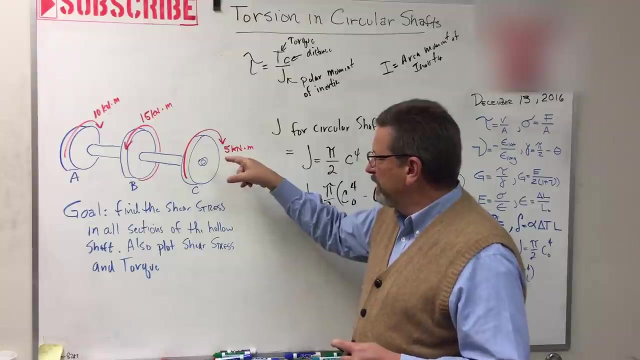 the fourth, I did it again inside. Sometimes my brain doesn't work good. Okay, so let's see if we can solve this problem with these two new equations. Okay, So I've got here. is this thing in equilibrium? Let's look at this. 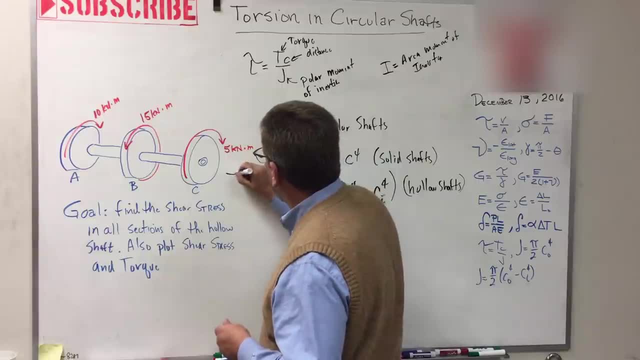 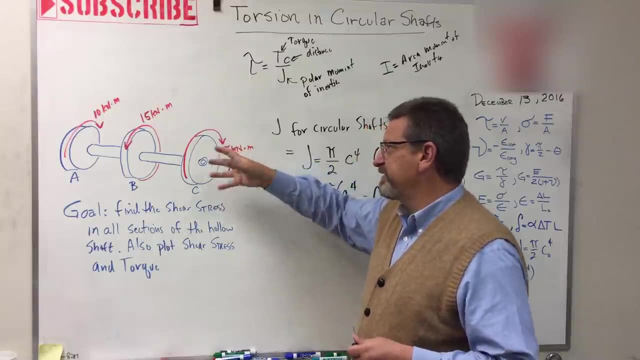 I've got a. what is that? If my eyeball is down here, right, here's your eyeball, okay, then that's clockwise, right, Okay? So I've got a clockwise, I've got a counter and I've got a clockwise. 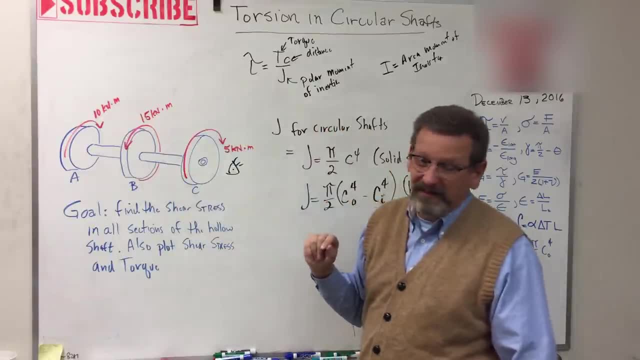 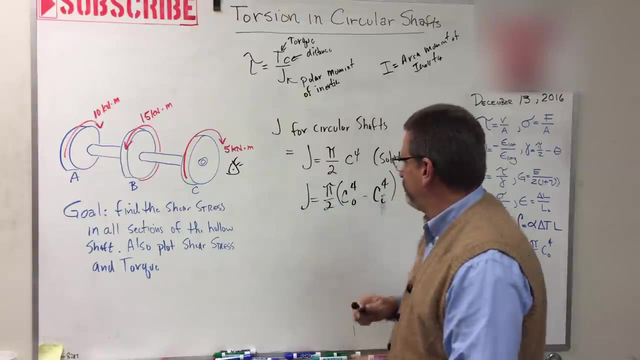 So my two clockwise ones are 5 and 10,, that's 15, and the counter is 15.. So the thing is in equilibrium right. It's just kind of hanging out there and it's got some torque applied to it. 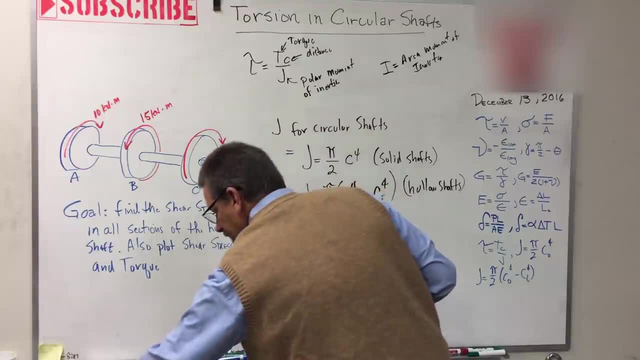 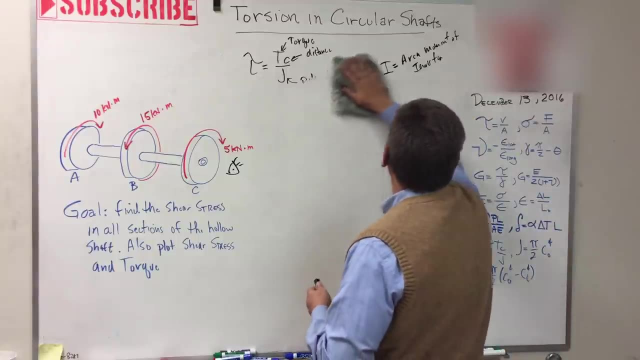 Okay, So let's see if we can do this. Okay, Erase, I'm going to erase. We've got all our equations written down. I'm going to erase everything here. okay, All right, here we go Now. this says: find the shear stress in all of the sections. 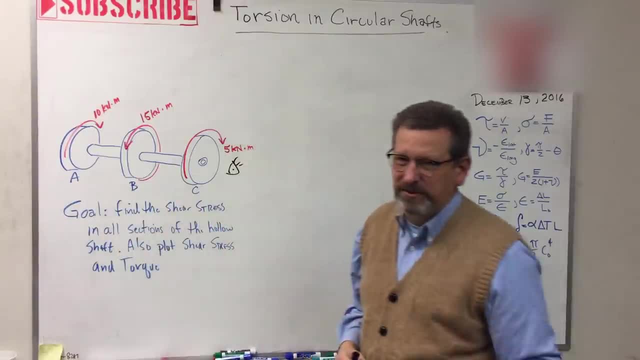 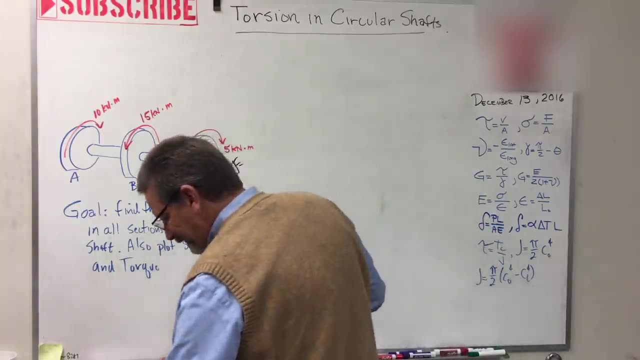 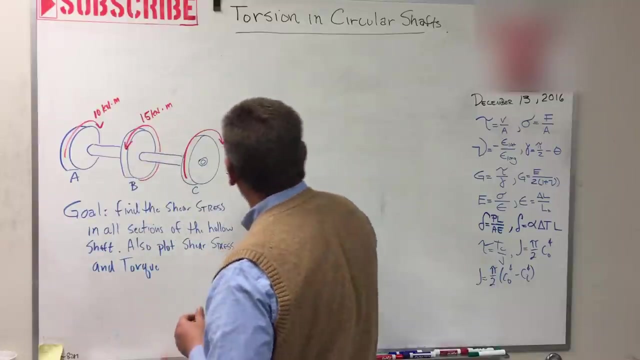 So we have section AB and section BC. There's only two sections Of the hollow shaft. I guess I should tell you, like, how big that is too. huh, I'm world famous about leaving dimensions off. It says that it's 180.. 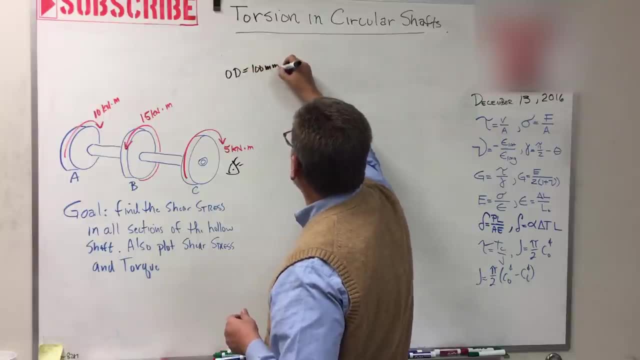 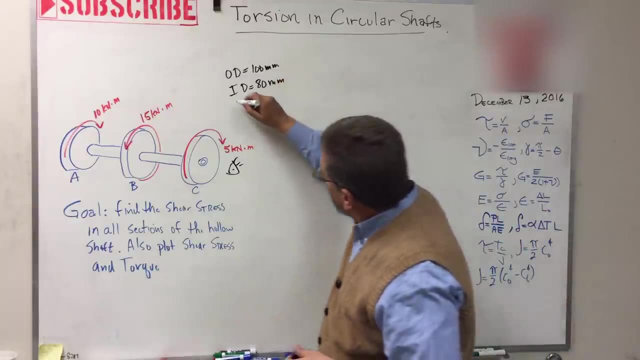 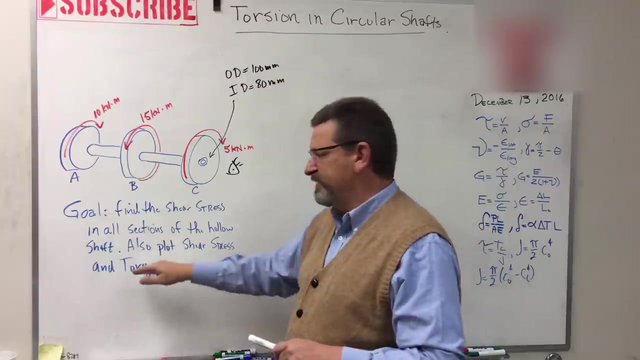 So OD is 100 millimeters, ID is 80 millimeters. okay, So we got that right. That's for that shaft right there. okay, So it says also: plot the shear, stress and the torque and let's do this okay. 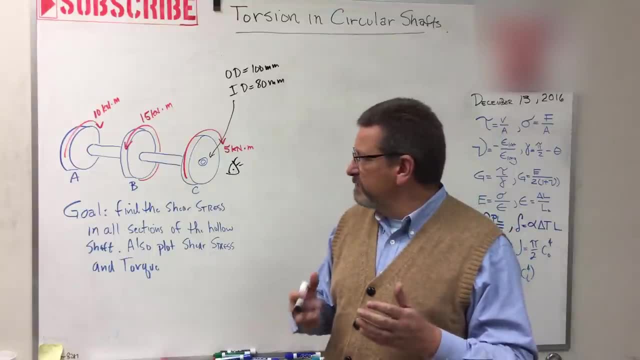 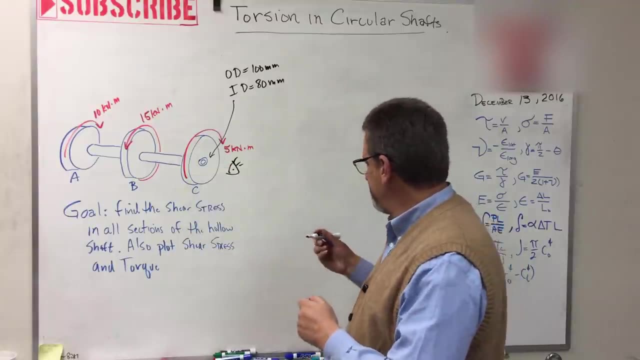 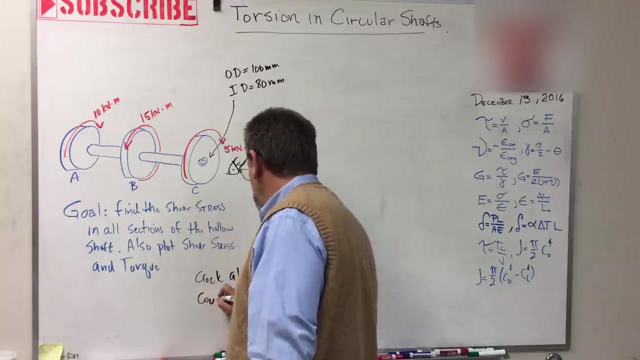 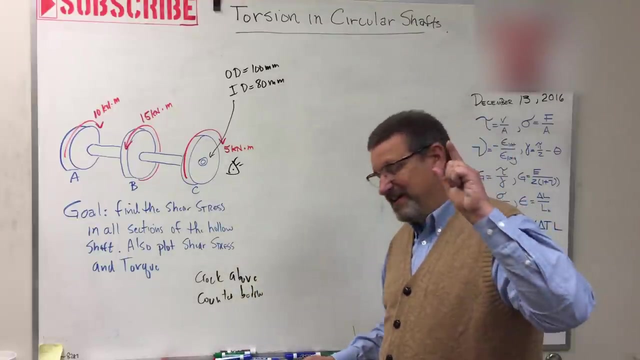 We're going to plot clockwise: Clockwise moments above the axis and counterclockwise torques below the axis. okay, So clock above, counter below. okay, How do you remember that? Here's how you remember it. Are you ready? 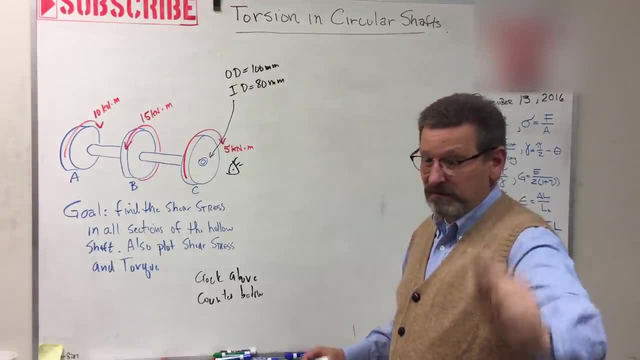 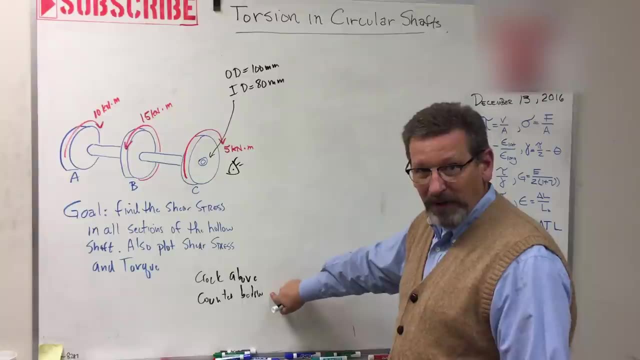 This is good. We're going to use this several times In the kitchen. the clock is above and the counter below Counter is below. okay, Clock above, counter below. Got it All right. We're going to use this a bunch. 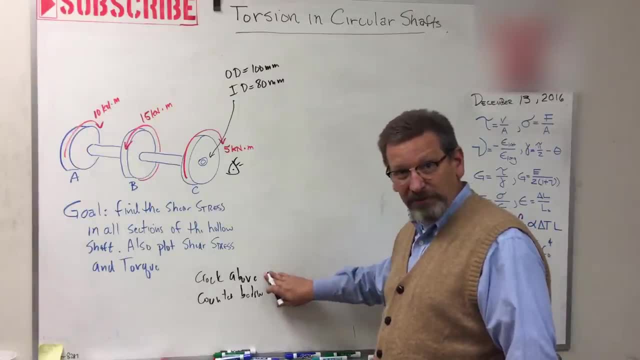 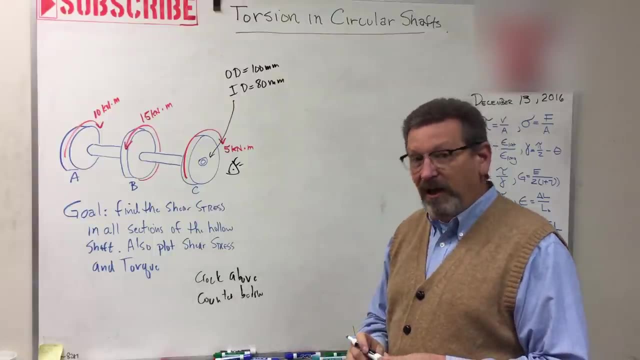 We use this when we do more circle. Same thing: If it has a clockwise rotation, I plot above the line. If it's counterclockwise, I plot below the line. So this is something to remember. We'll use it again, okay. 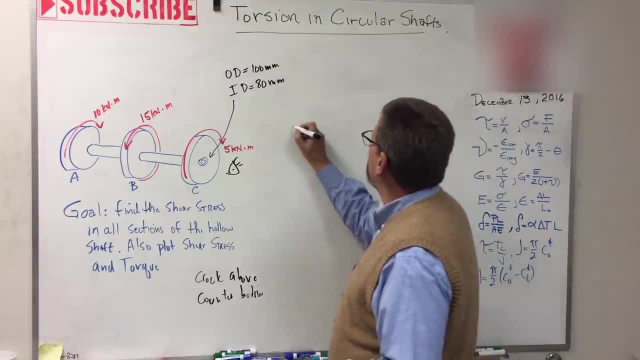 Clock above in the kitchen, clock above counter below. All right, here we go. So first let's just do torque, okay. So here's point. let's say here's point A, Here's point B And here's point C, okay, 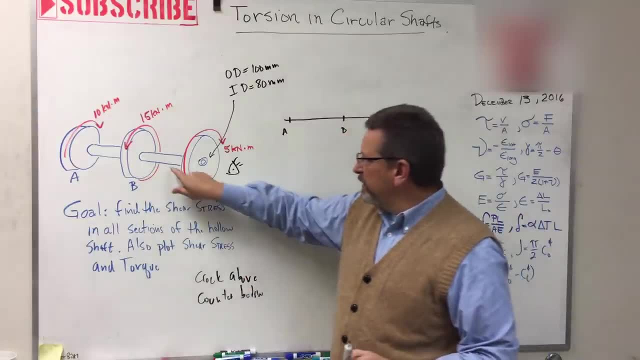 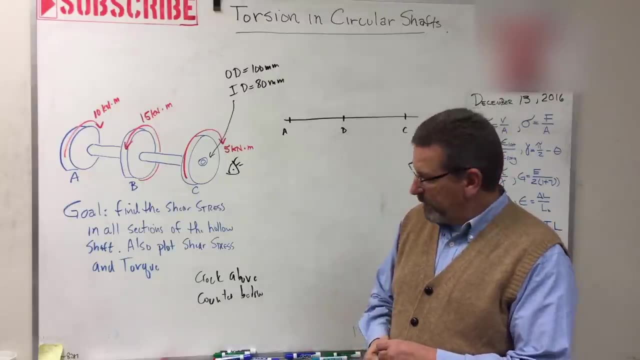 Let's start with this section down here. B, C, This section of the shaft, is it feeling a clockwise torque or a counterclockwise torque, And how big is it? Well, how do I tell? I don't even know. 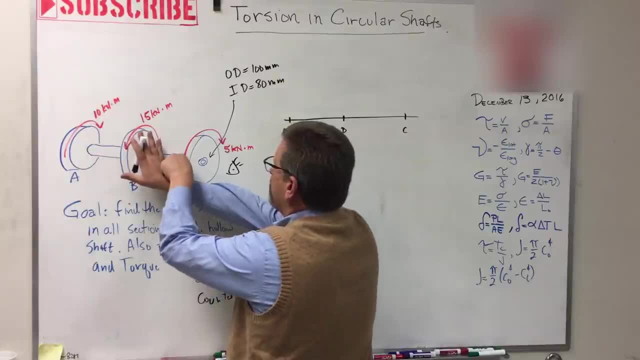 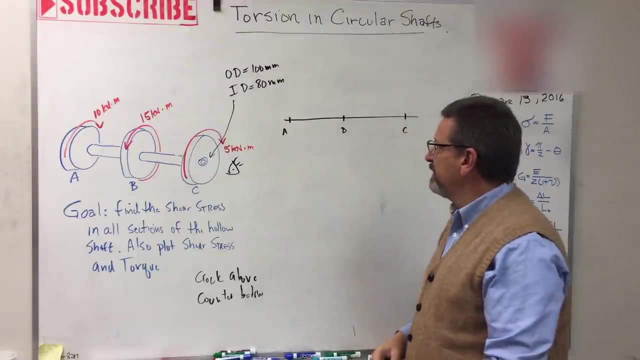 Here's how you tell: Just cover all this up. So what is this shaft? If I just cut it right there, what's it doing? This thing has got a clockwise torque on it, doesn't it? Okay, So this section down here is clockwise. 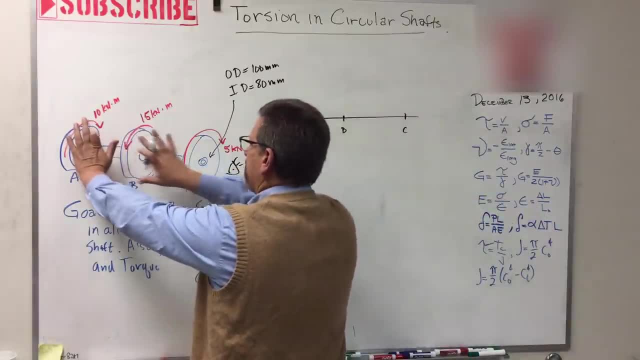 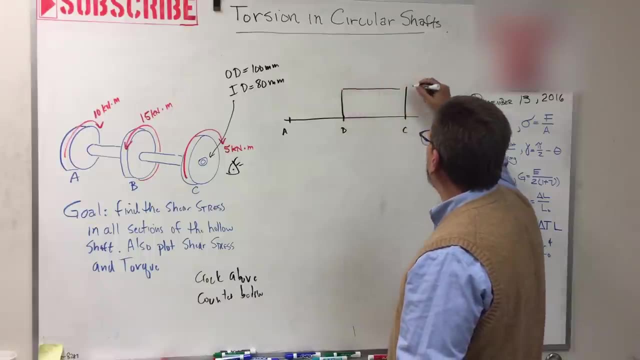 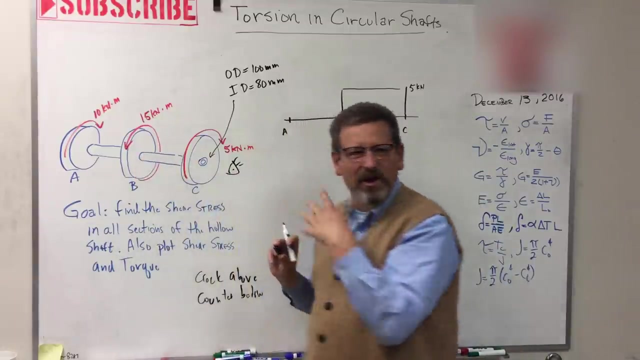 And how big is it? How big is the torque in this section down here? It's clockwise and it's five kilonewtons, right. So here we go, whoop five kilonewtons, And that torque is from right behind this to right there, right? 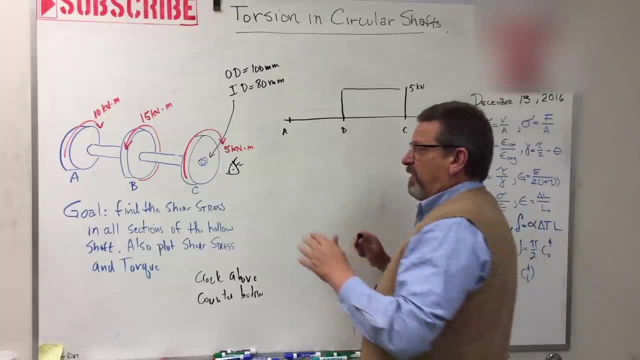 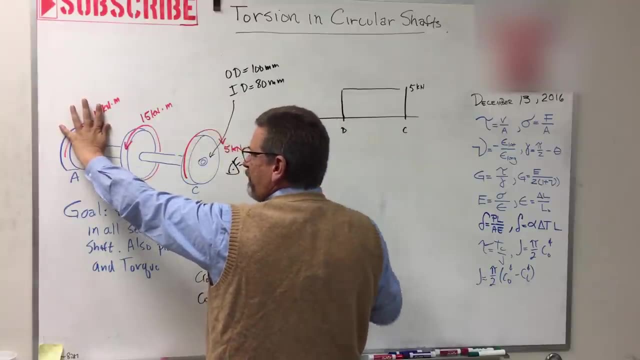 The whole shaft has the same torque in it. okay, What about on that end? What if I cover that up? What about on this end? I've got five clockwise and 15 counterclockwise. Okay, I've got 15 counter. so that nets me what. 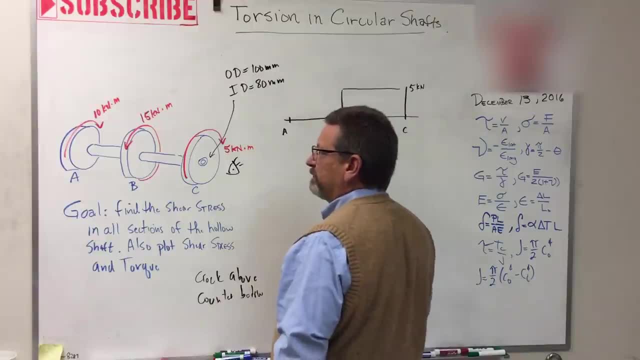 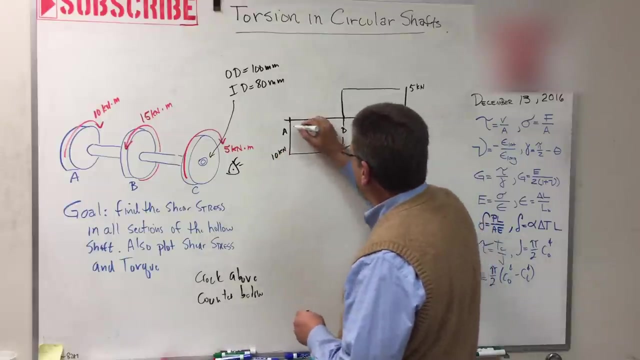 That nets me 10 counter, right, Right. So 10 counter it goes the other way, doesn't it? This section down here has 10 kilonewtons, okay, So that is the amount of torque in those sections of the shaft, okay. 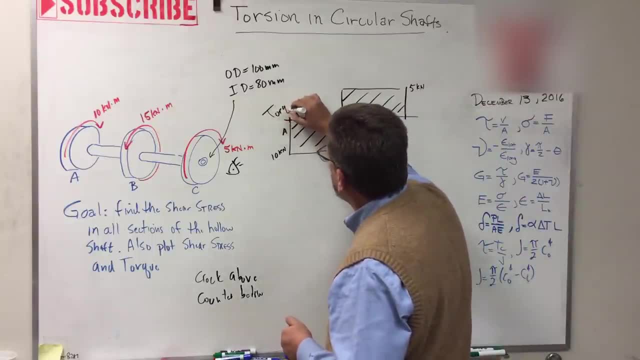 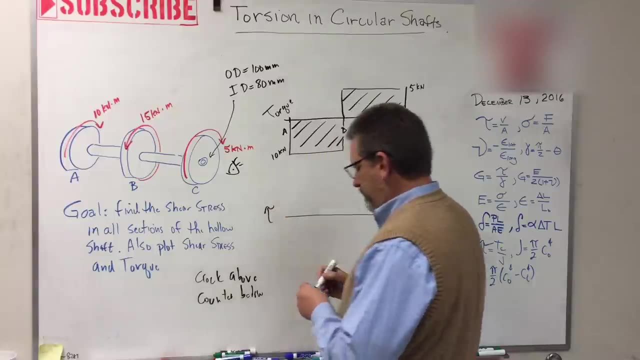 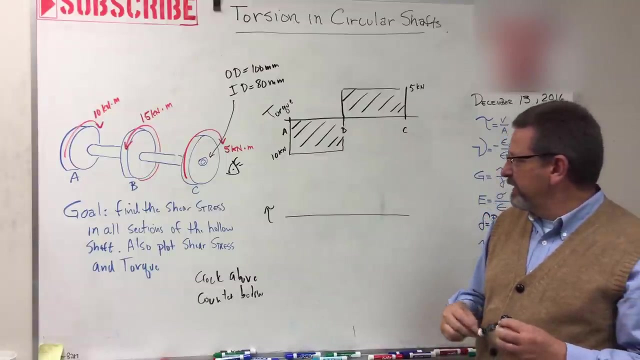 This is a torque graph- T-O-R-Q-U-E. okay, So how can I find out what the tau is going to be for those graphs? What's that going to look like? okay, Now, it's not really that important to put the shear stress direction on here, because 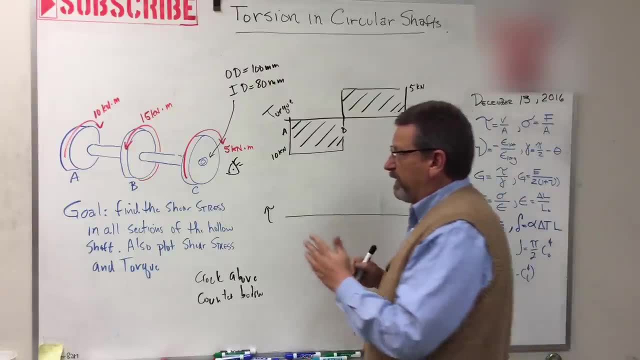 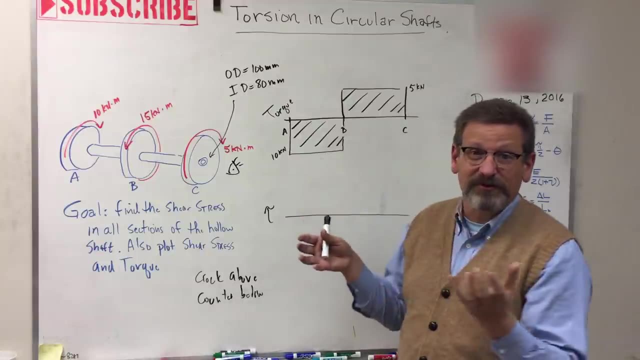 shear stress. think of it as an absolute. because if I think about, if I cut that shaft, one side the shear stress is one way, but on the other side of that cut, the shear stress is the opposite way. So you really 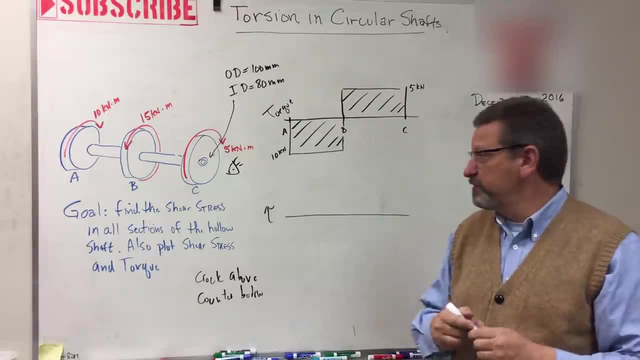 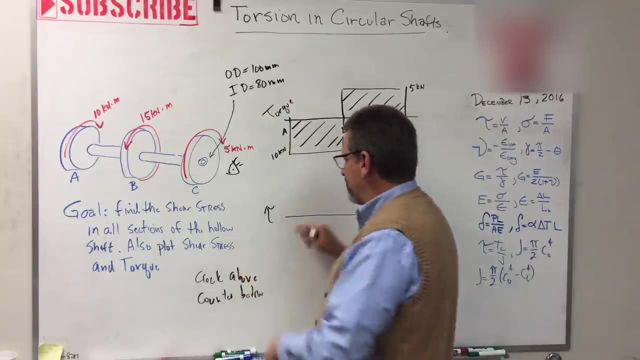 As engineers, we're worried about the absolute value of that shear stress and what it is okay. So how do I find out what the shear stress is? Now, when it says plot shear stress, is that going to be a curvy line? 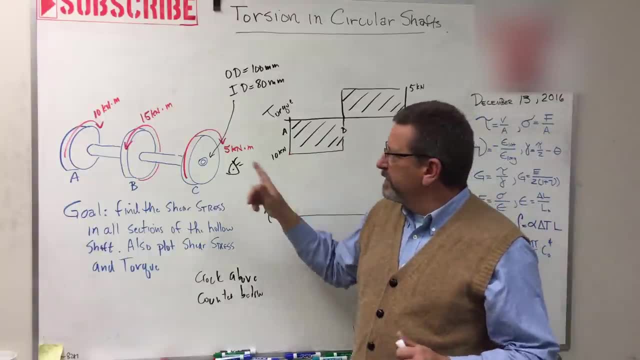 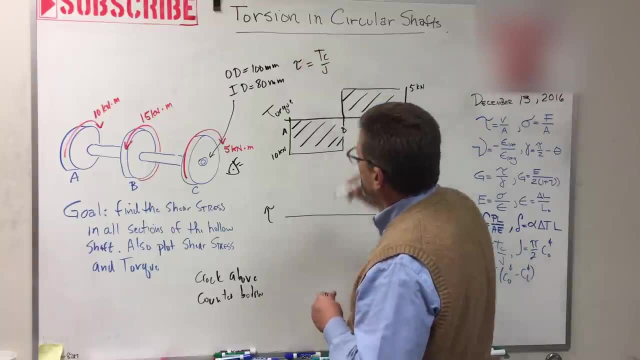 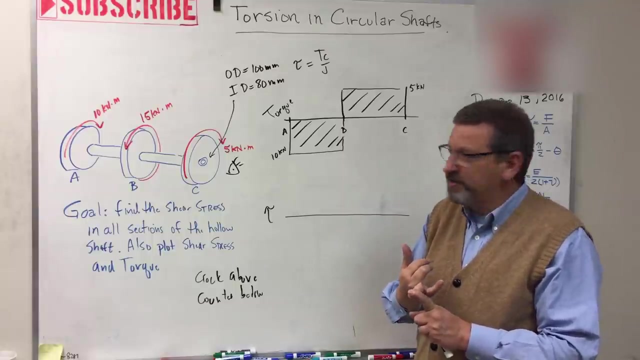 Well, let's think about from A to B. okay, Let's think about that. Our equation is this: right, Our equation is T-C over J. okay, There's tau. So T is constant. Is C constant? Yeah, The radius or diameter never changes, does it? 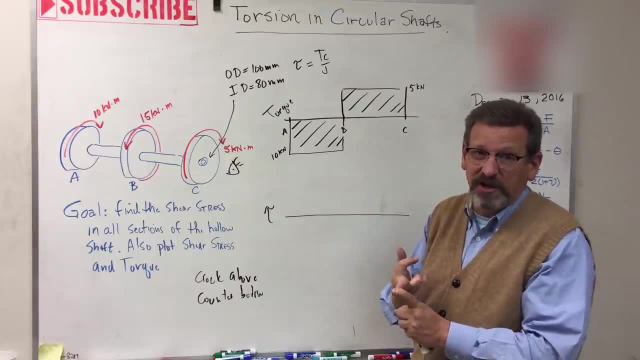 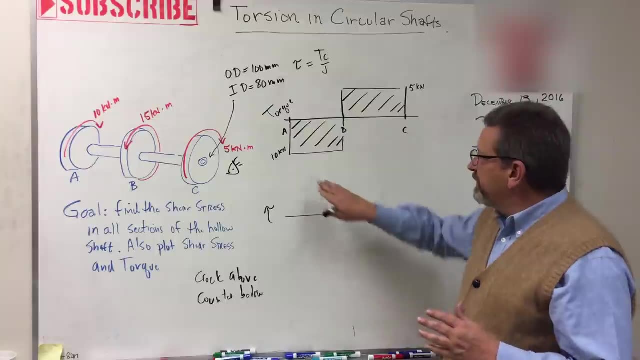 Is J constant? Yeah, The polar moment of inertia is constant, right, Because there's the equation for it, right there. C never changes and pi doesn't change, So it's going to be a constant shear here and then a constant shear there. 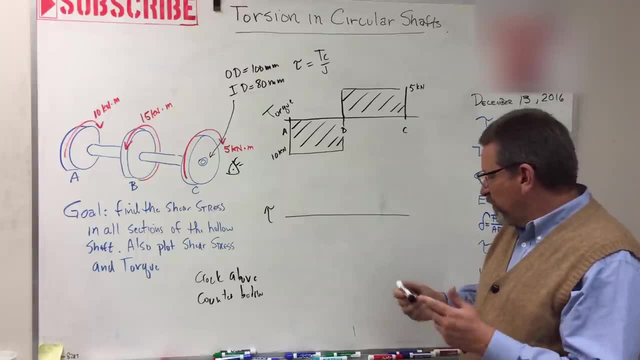 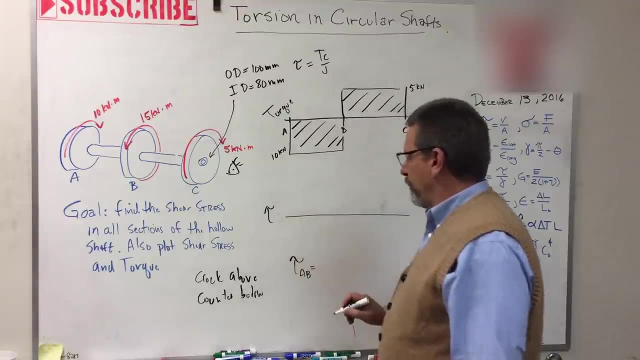 It's going to be two different values, but it's constant in both places. So all we got to do is calculate what it is. So let's do: tau A to B is equal to the torque. That's easy right. That's T-C over J, Okay. 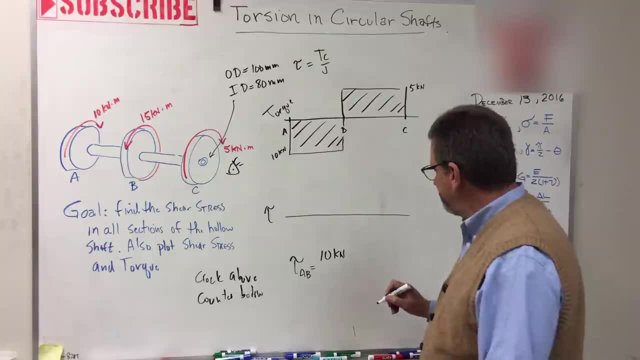 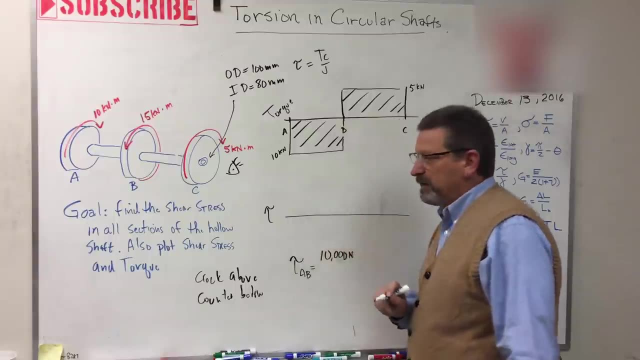 10 kilonewtons. Now we're going to be really careful with our units, right Matter of fact, let's do this. Let's do 0, 0, 0 newtons, because if I get newtons over millimeters, that's what. 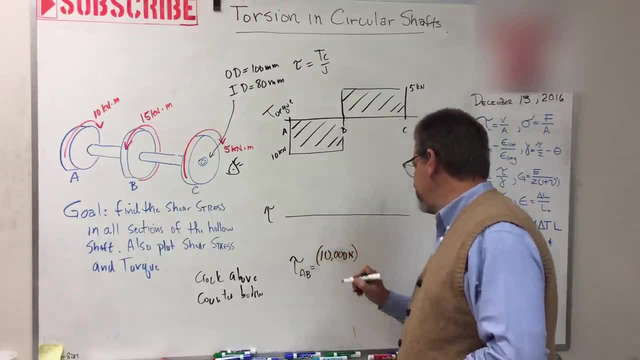 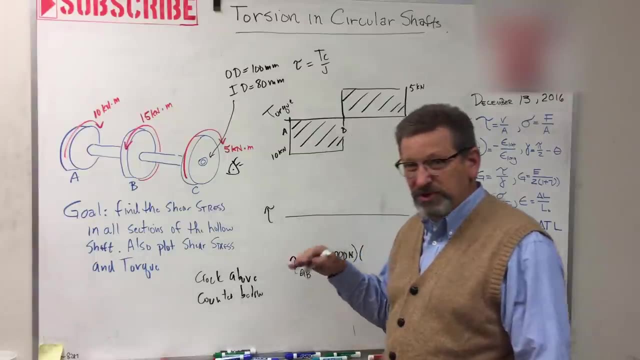 That's megapascals, right? So let's put it in a unit we know. So 10,000 newtons times C, all right, C is we're going to have to find the maximum shear stress which is going to be at the. 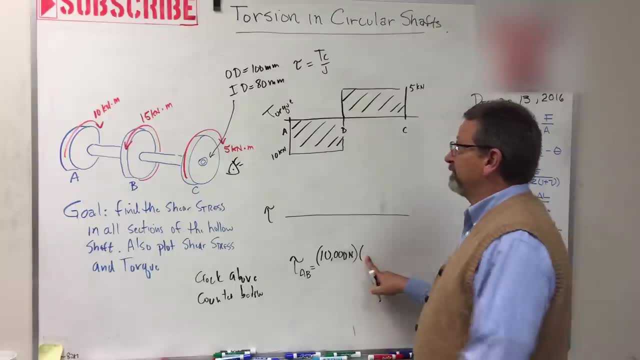 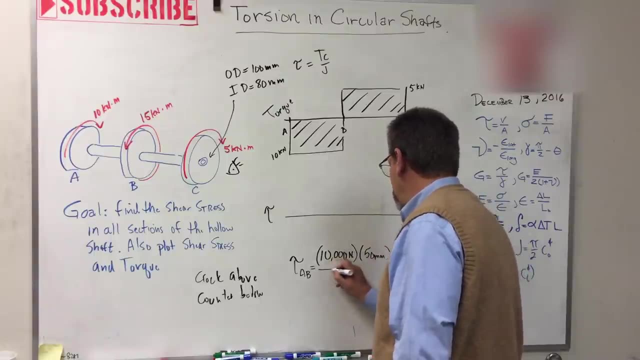 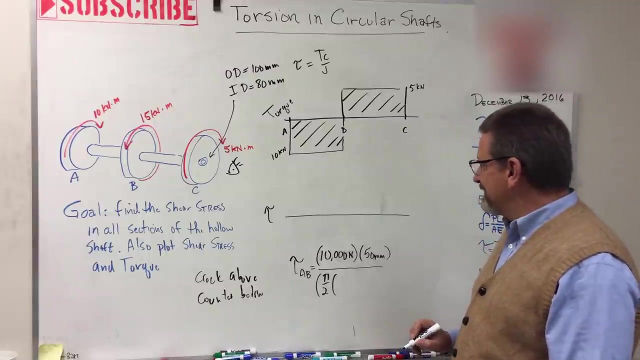 outside of the part. And so what is C going to be Half of the big value, right, The OD. So 50 millimetres, okay, divided by J. Okay, here we go. So J for this guy is going to be pi over 2 times the outside radius, which is what 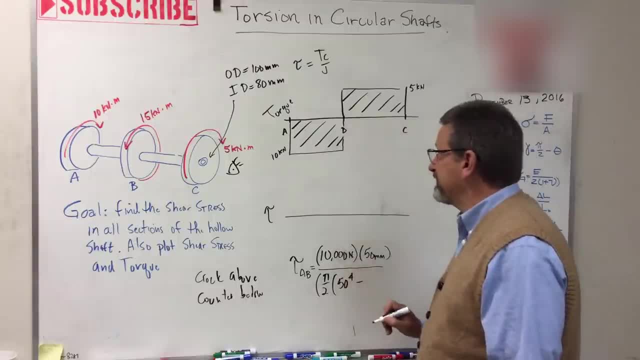 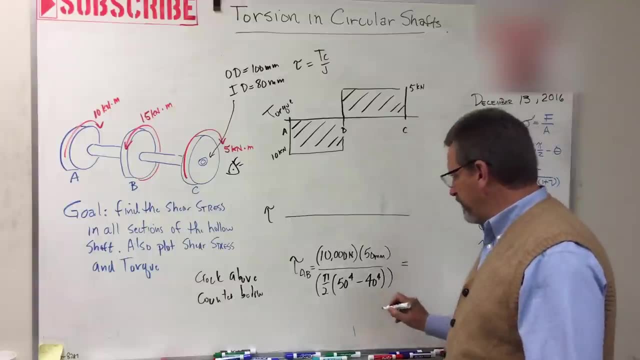 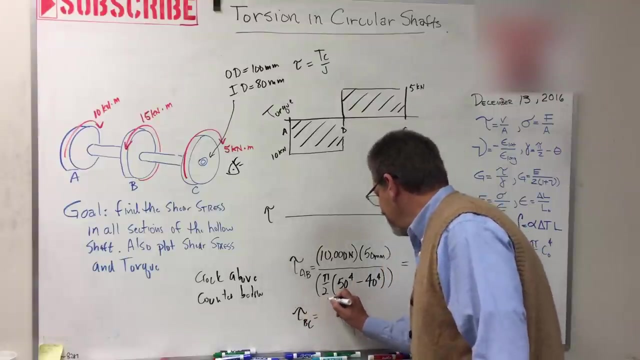 50 to the fourth, minus the inside radius, which is 40. Okay, And there it is right. Now we can do the same thing down here for tau. what is it? BC, Tau, BC. what's different? The only thing different is the torque on it is 5 kilonewtons. so that's going to be. 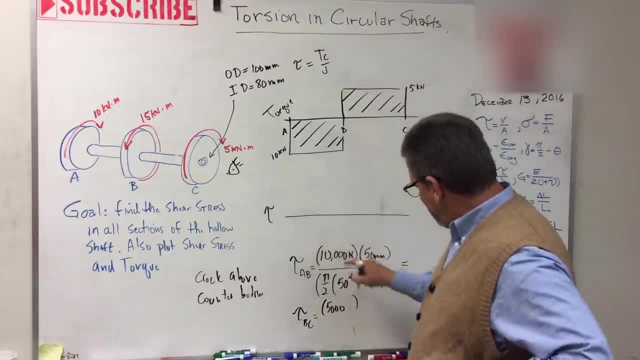 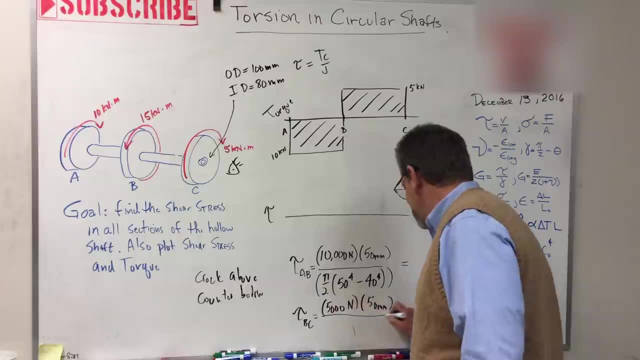 5,000.. I think that's going to be half of that. what do you all think? That's newtons times 50 millimetres. It's the same size OD And it's the same J. Is that right? 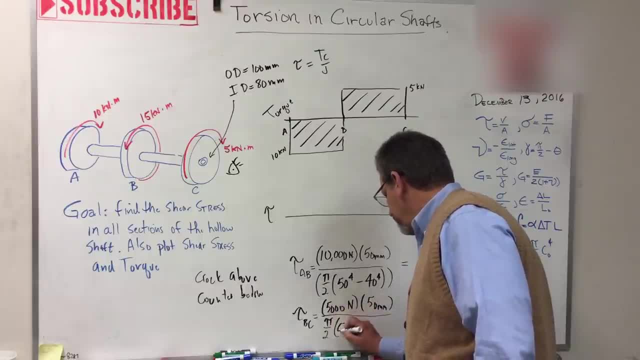 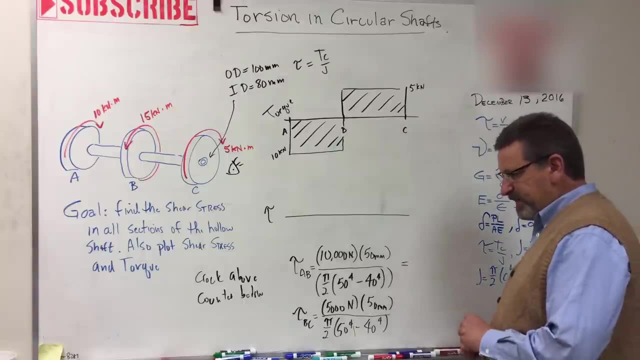 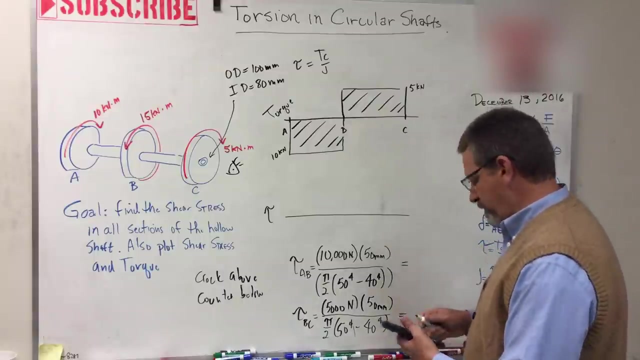 It's the same J, isn't it? Pi over 2,, 50 to the fourth minus 40 to the fourth. Okay, Let's see what we get. It's calculator time, Okay, here we go. So I have, let's do that bottom down there, right. 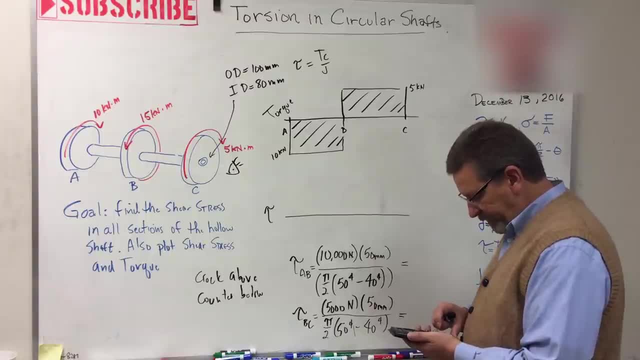 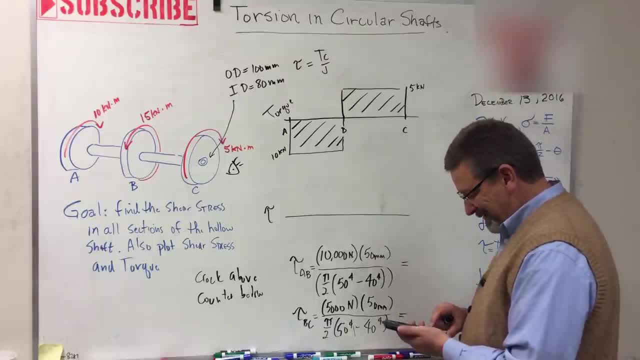 50 to the fourth arrow over minus 40. to the fourth arrow over minus 40. to the fourth arrow over minus 50.. Okay, equals, times, times pi, times pi, equals. divided by 2, equals. okay, and then I've.